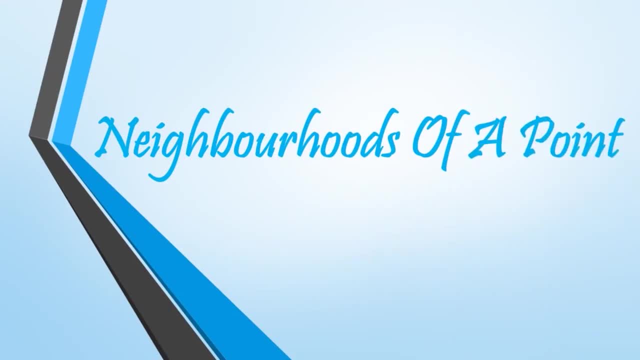 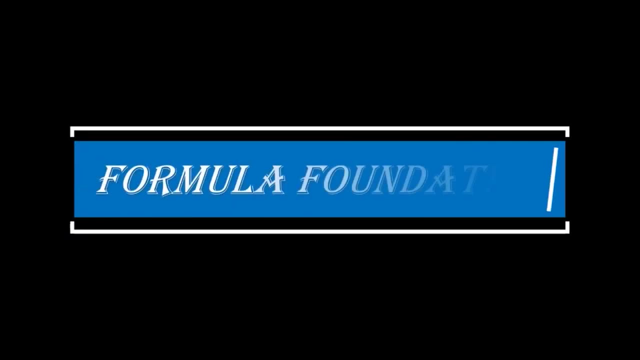 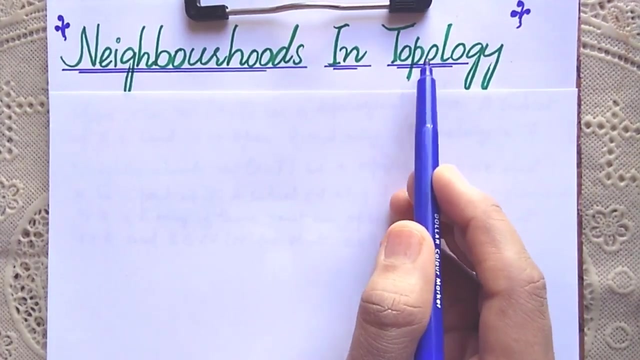 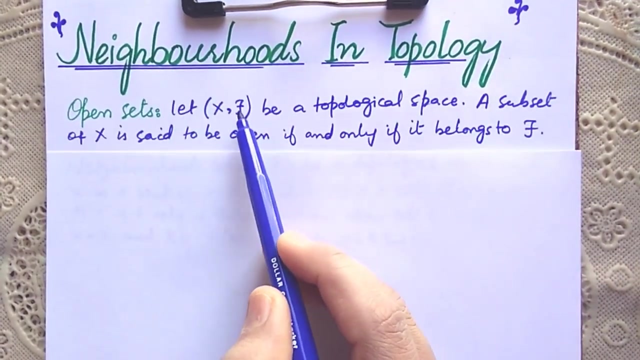 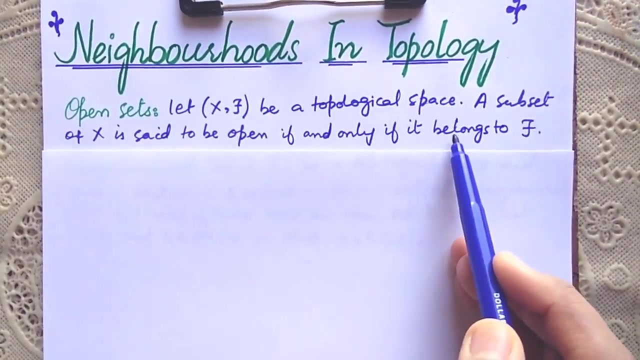 Welcome to the Formula Foundation Neighborhoods in topology. Before starting the neighborhoods, you must aware about open sets. So what are open sets? Let x with the topology tau be a topological space. A subset of x is said to be open if, and only if, it belongs to tau. Right. 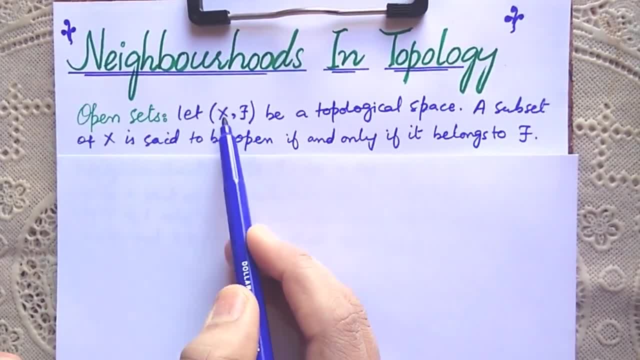 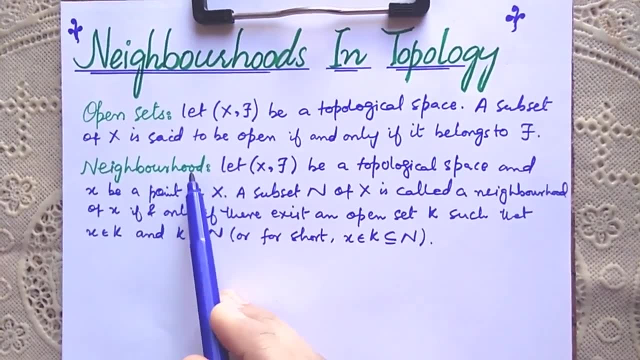 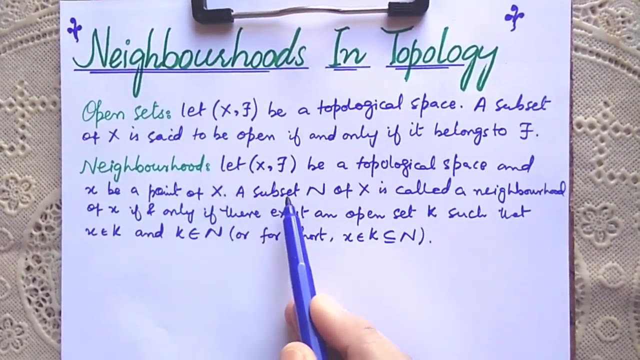 Means ground set x ke wo subsets open sets ke laayenge jo topology tau se belong karenge. Right Now let's start neighborhoods. So here is a formal definition: Let x with topology tau be a topological space and x be a point of ground set x. A subset n of x is called a neighborhood of x. 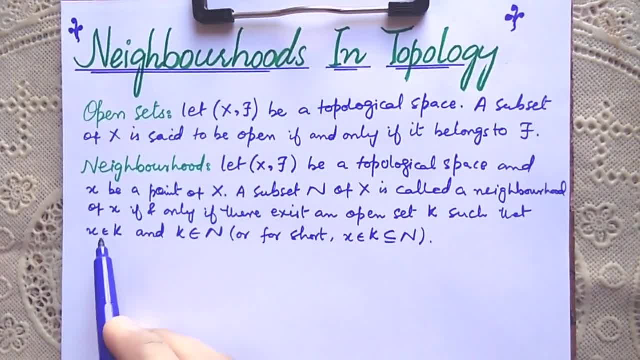 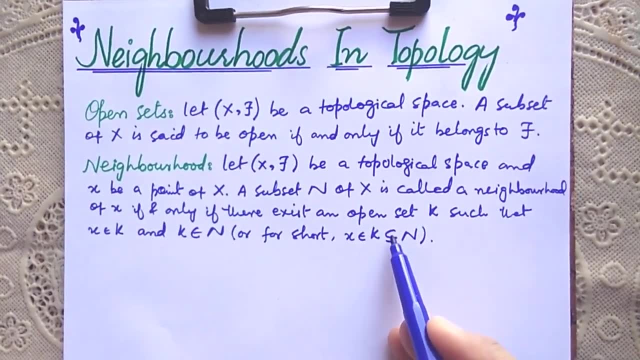 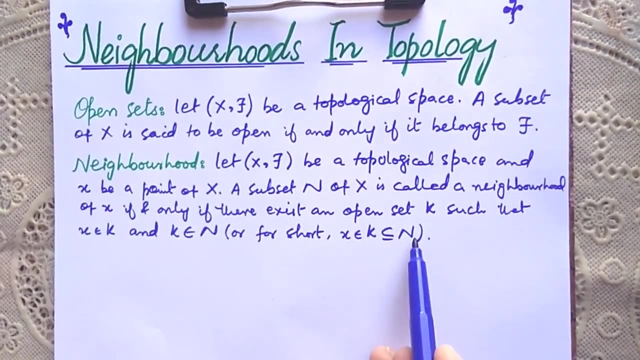 there exists an open set k, such that x belongs to k and k belongs to n, or, for short, x belongs to k and k is the subset of n. Right Means neighborhood. x set hai Set n Aur wo kisse associate kar raha hai. 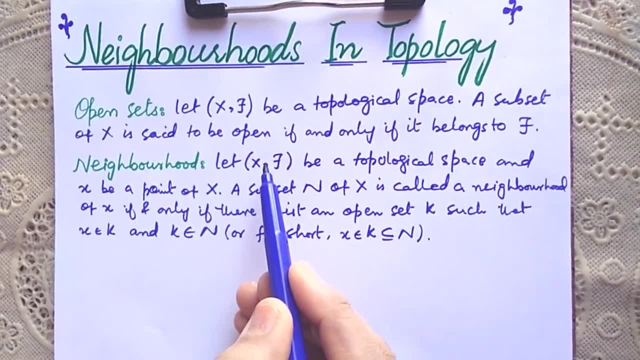 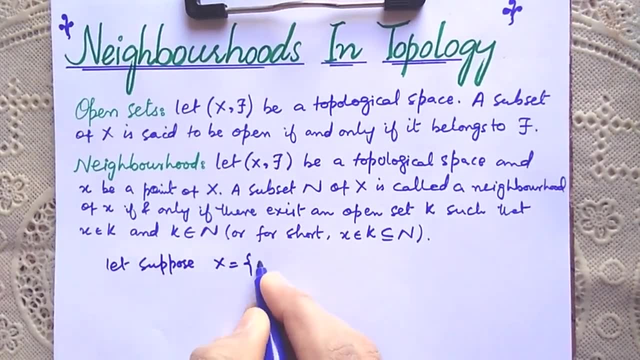 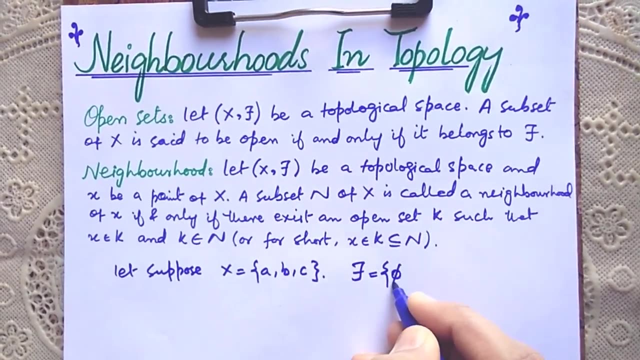 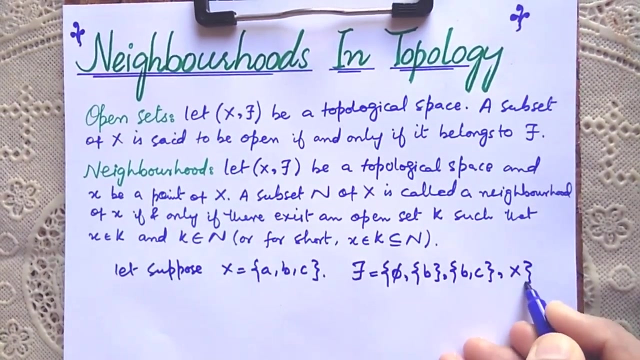 Ground set ke ek point se Right. So let's suppose ek set hai. Let's suppose ek ground set hai x is equal to c and there is a topology tau, let's say phi, b, bc and x, Right. So ab neighborhood x ke har ek individual. 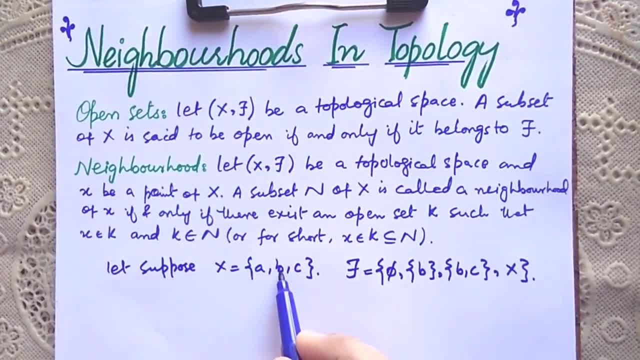 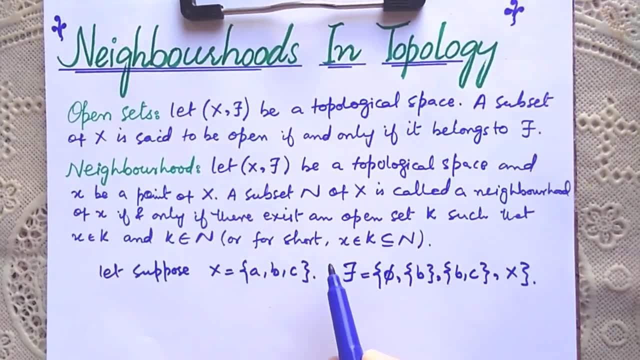 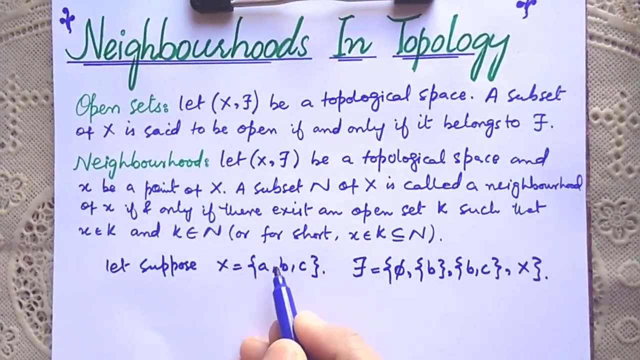 point ke liye find karenge Means neighborhood of a, neighborhoods of b and neighborhood of c. And what is neighborhoods? These are subsets that satisfy some specific conditions, Aur wo conditions kya hai? So hum ek point lete hain, x mese. Let's say wo point hai a, And for better understanding, hum x ke. 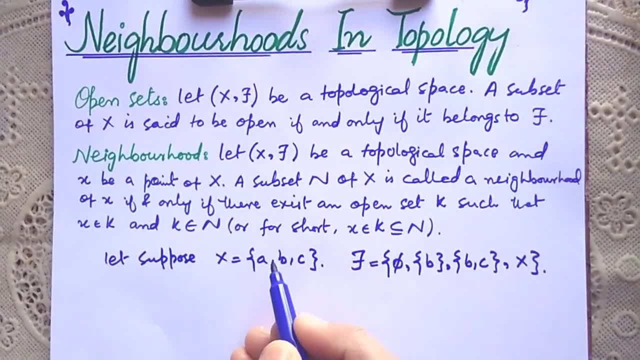 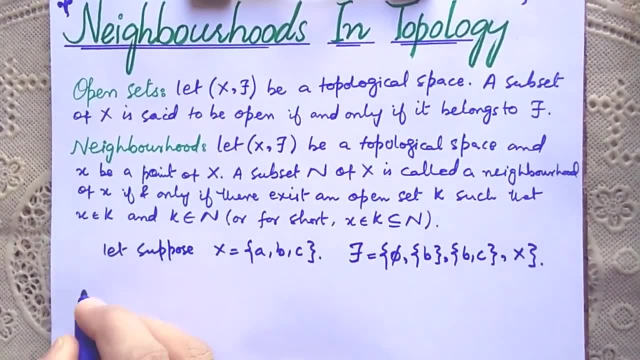 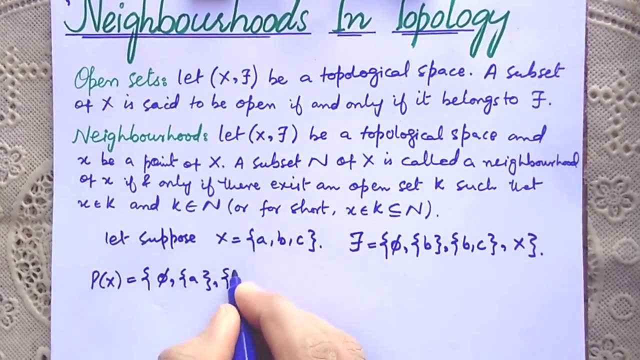 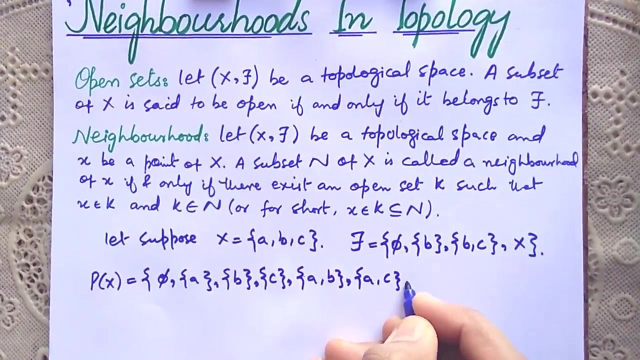 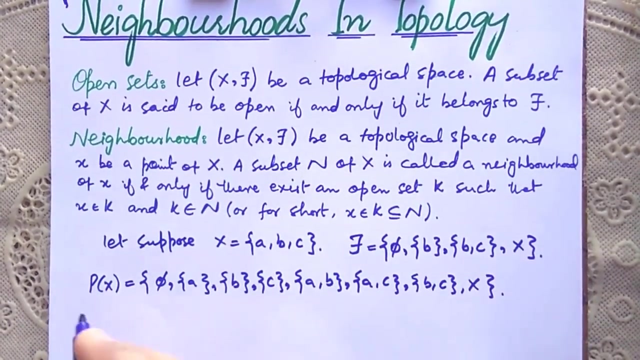 tamam possible subsets likh lete hain, Because again I am repeating neighborhoods of a point. are these some subsets of x that satisfy some specific conditions? Right? So all possible subsets of x are phi, a, b, c, ab, a And the C and b, C and the whole x Right joints ut ki b, c ride. Now we have to find we 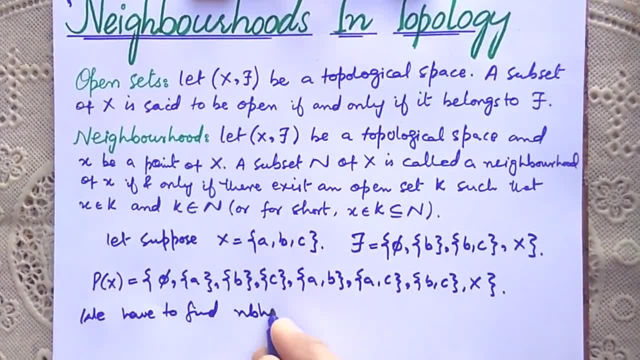 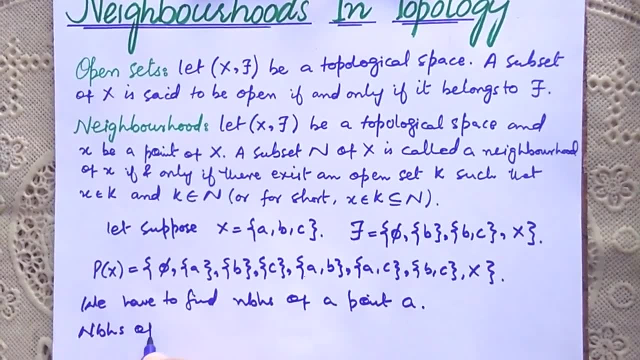 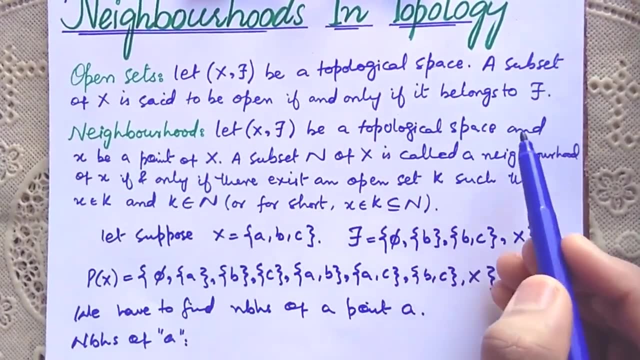 have to find. Well, you canственный abg und a right Neighborhoods of a point, a Right Neighborhoods of a. Now again with the definition, let x with topology tau each topological space, x be Labs o obve doformule space and x be a point of x. N ab kic Wisconsin, toh, bah, noisy lady. 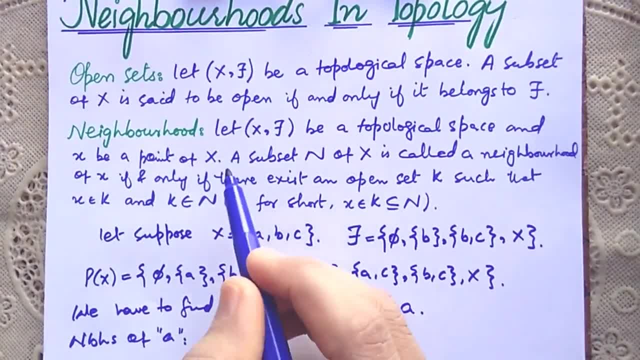 point of x di barri. Now here a point of r x. toh unit Ni barare r x offering R o I. yeah, ok, So a plate, t rub A plate and tohe r here. x is a right, a subset n of x is called a neighborhood of x if, and only if, there exists. 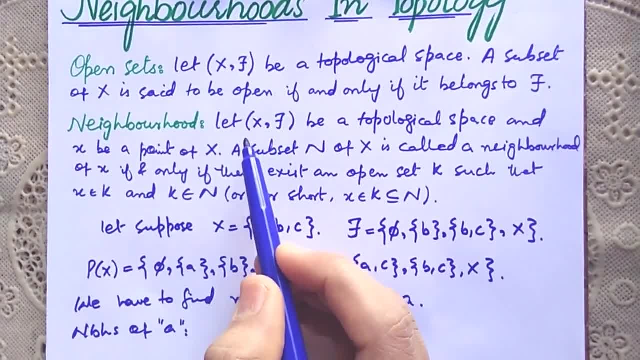 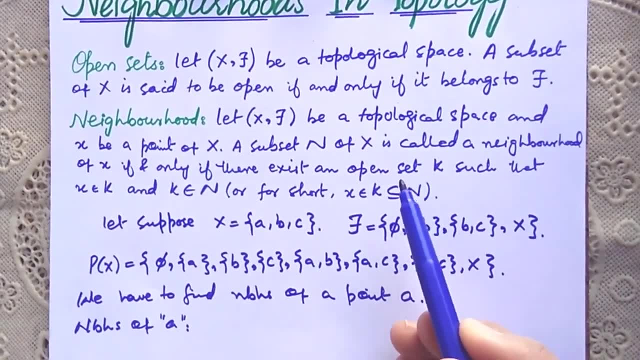 an open set k means x ka koi subset a ka neighborhood hoga. akar koi open set k exist karta hai. yaani tau mese koi ek set k exist karta hai, such that a uss set ka member hai, means x belongs. 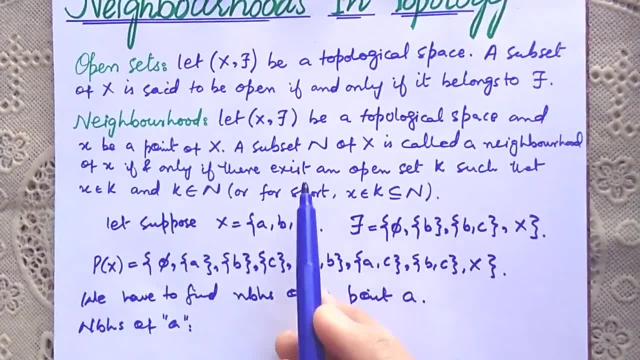 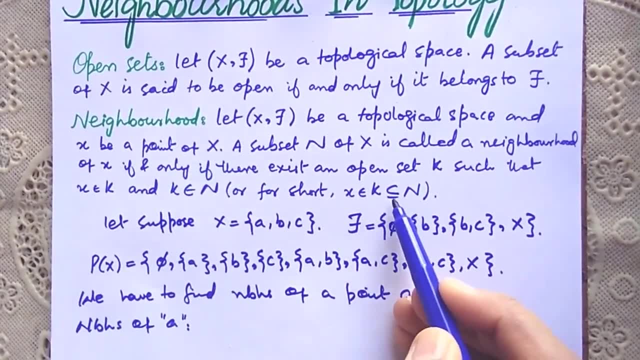 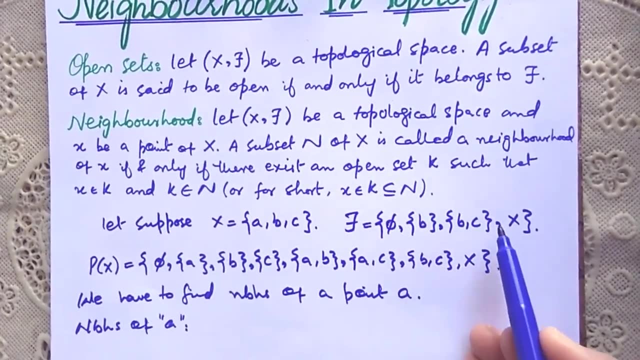 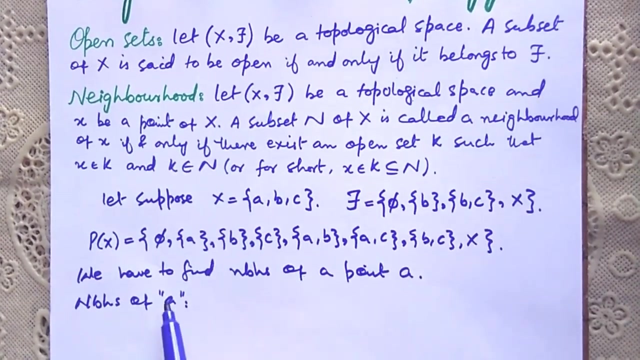 to k aur a belongs to k right and k x k kisi bhi subset ka subset ho means x belongs to k and this open set k is the subset of n right means agar ab hum tau me dekhen to there exist a subset. x means x is open set right and a belongs to x. so here k is equal to x right. 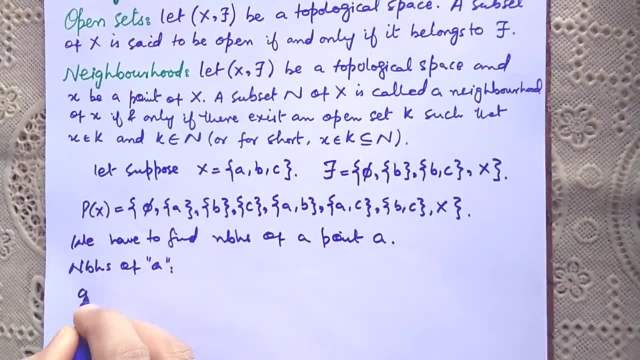 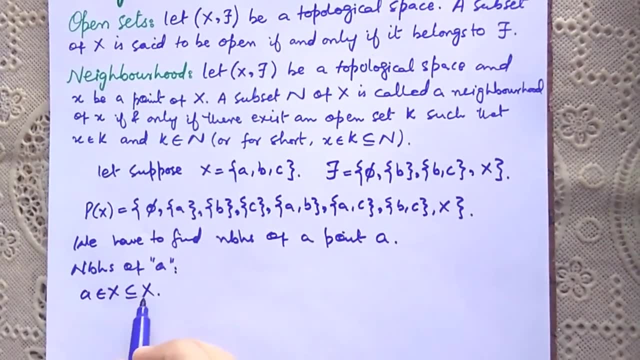 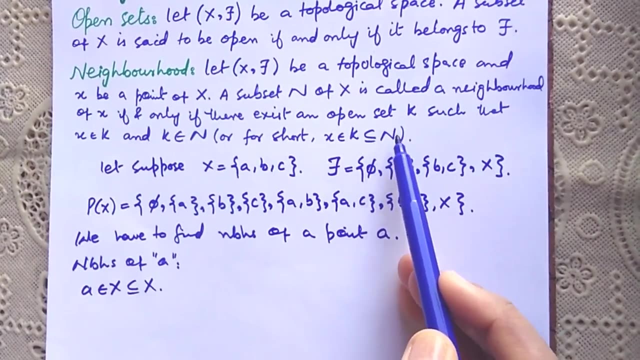 and a belongs to x, So a belongs to x, So a belongs to x. So we write a belongs to x, such that a x is a subset of itself. right means x jo subset x hai. wo is condition ko satisfy kar raha hai? x belongs to k and k is a subset of n. 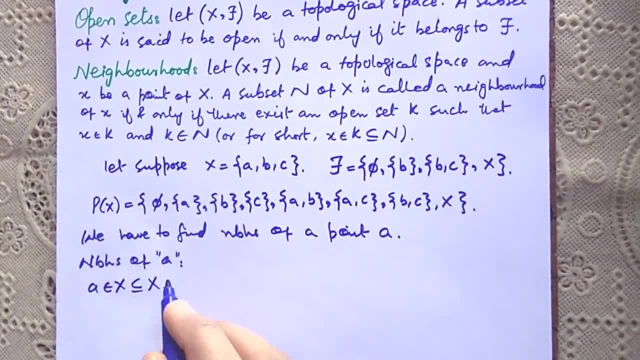 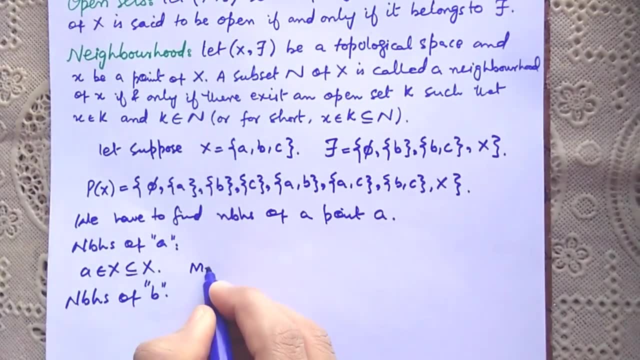 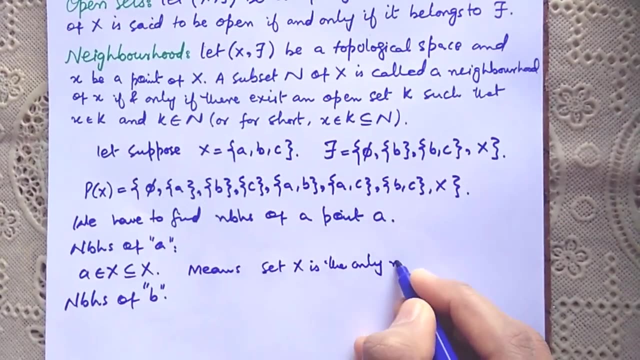 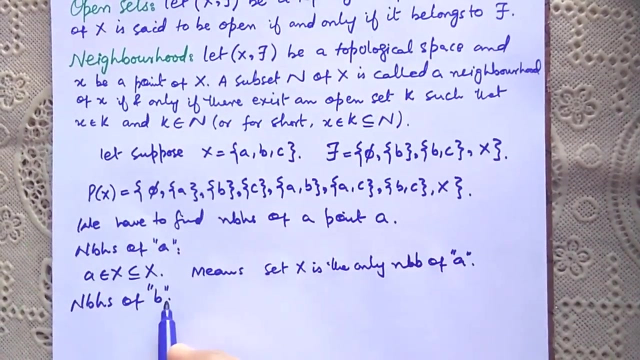 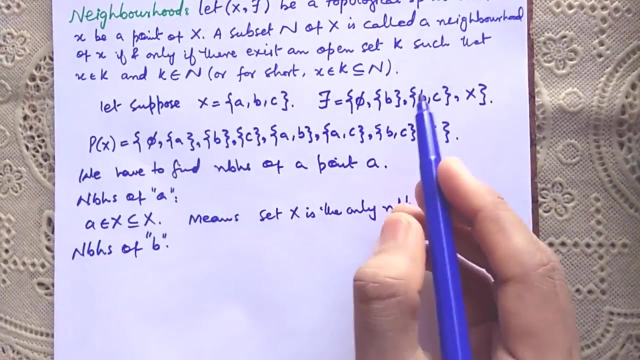 means x is a neighborhood of a right now. neighborhoods of b. point b means set: a is a. x is the only neighborhood of neighborhood of point a right now. neighborhoods of b. now is there exist a subset in tau such that b belongs to that subset. so yes, there is a subset. 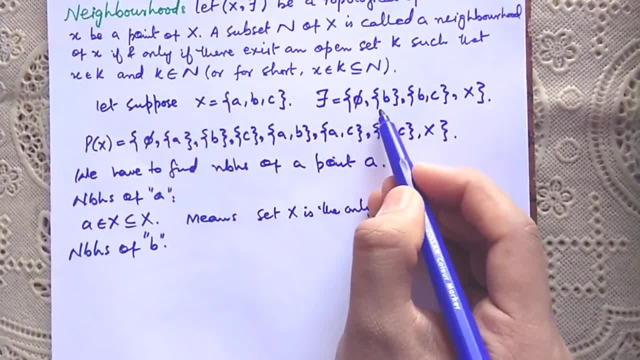 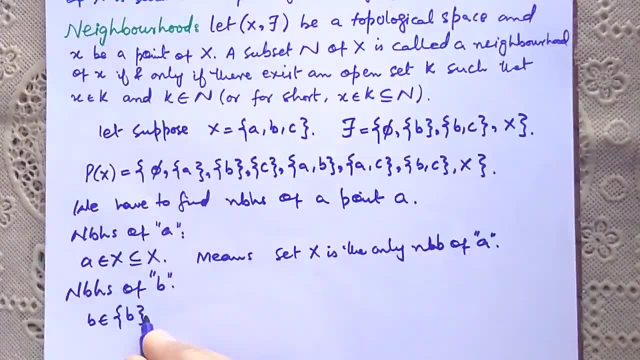 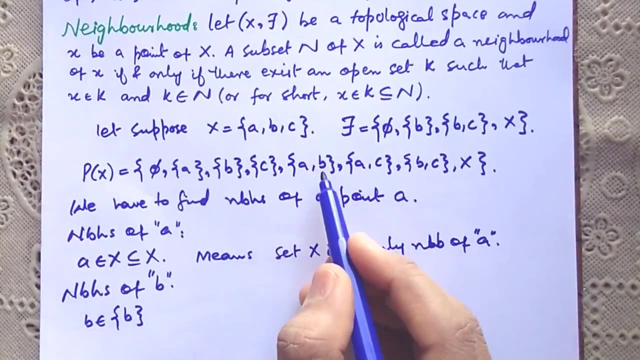 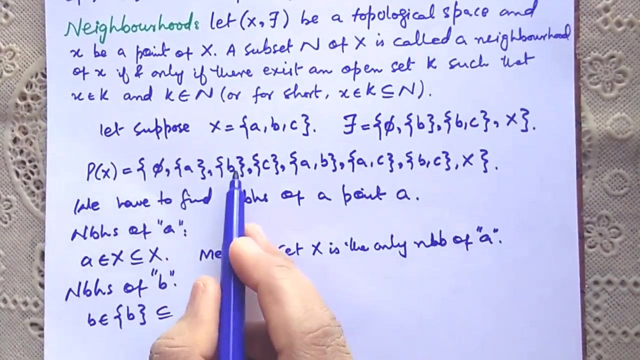 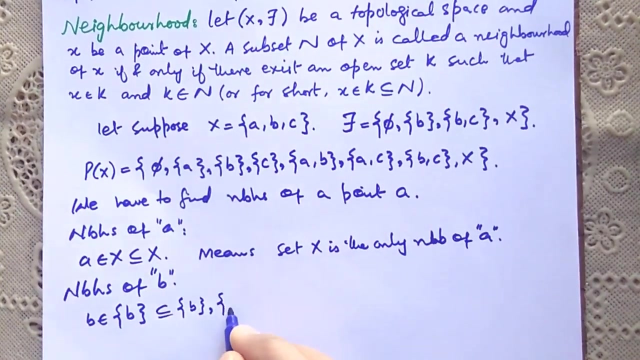 b in tau, such that b belongs to this set, this open set b. so b belongs to b right and groundset. mein se koi aisa subset hai jiska b subset ho, yes, there exist a subset that are supersets of b, that is: b is the subset of itself, b and b is a subset of. b is a subset of ab and b is. 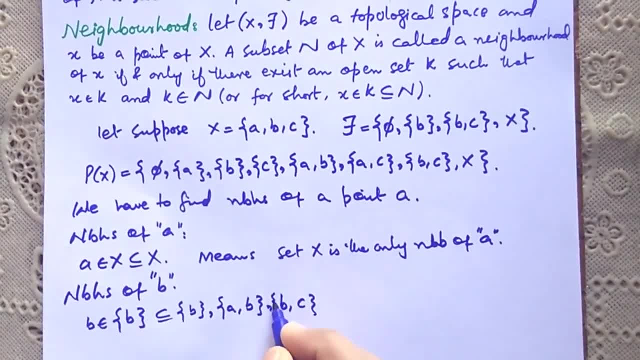 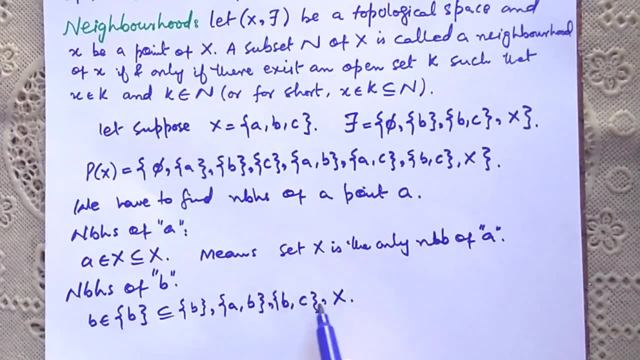 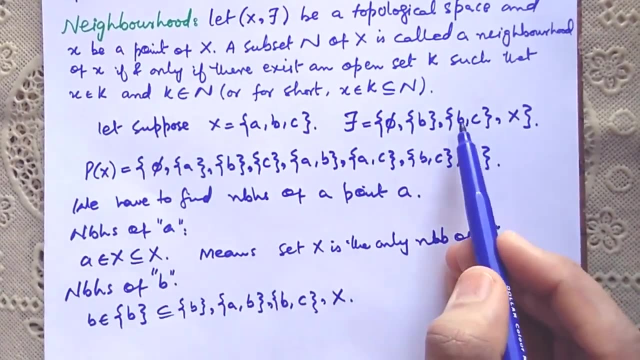 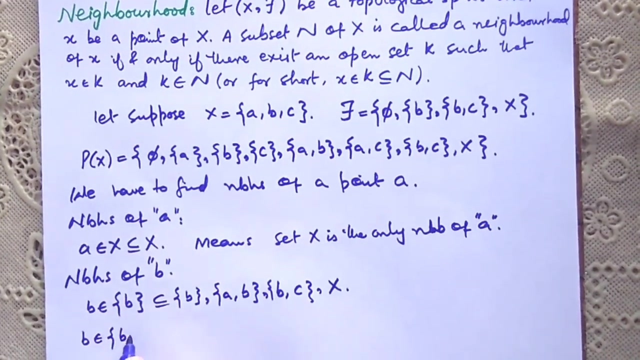 a subset of bc and also b is the subset of groundset. So this is a subset of groundset. x, right, so these are the neighborhoods of b. now notice that again there exist an another open set in tau bc, such that b belongs to bc. so here b belongs to set bc, and there are 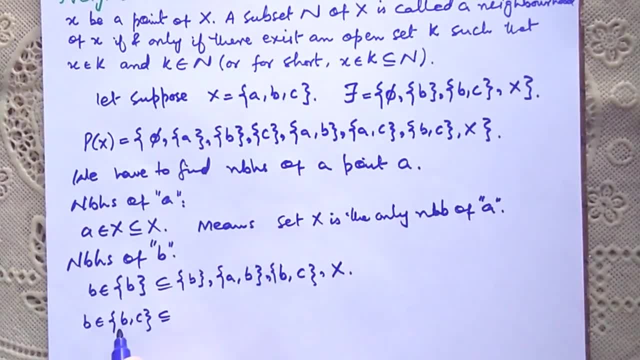 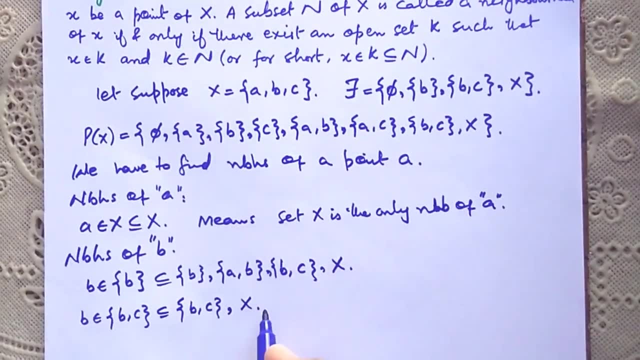 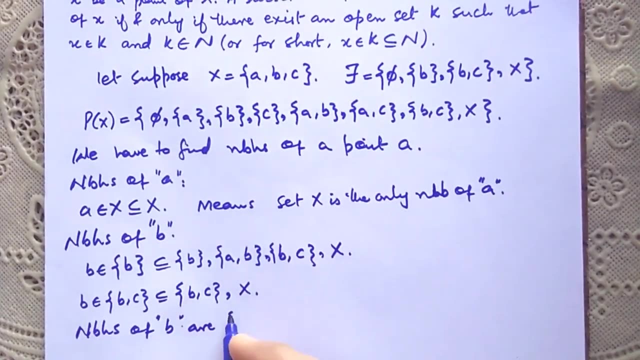 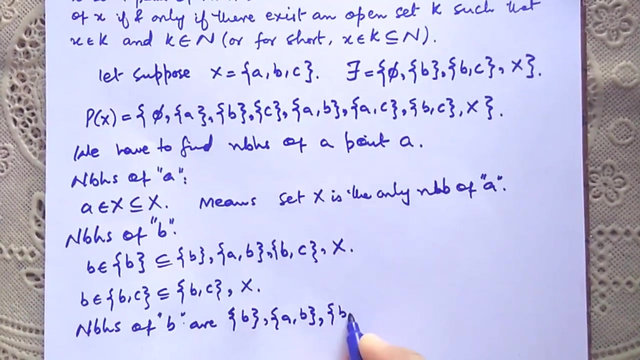 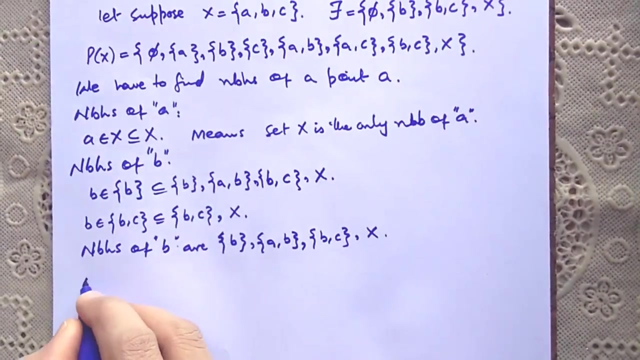 subsets in a, in a groundset, x, such that bc is the subset of bc itself And only x. right? so neighborhoods of b are neighborhoods of b, are b itself, ab, bc and bc and x right now. finally, neighborhoods of c: Right, Right Right. 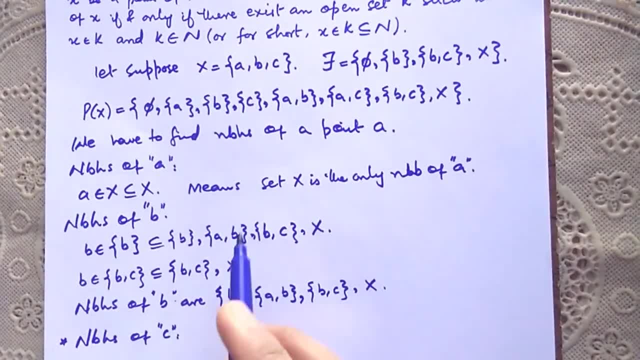 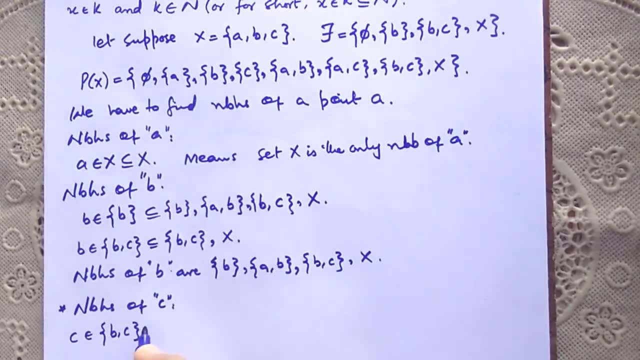 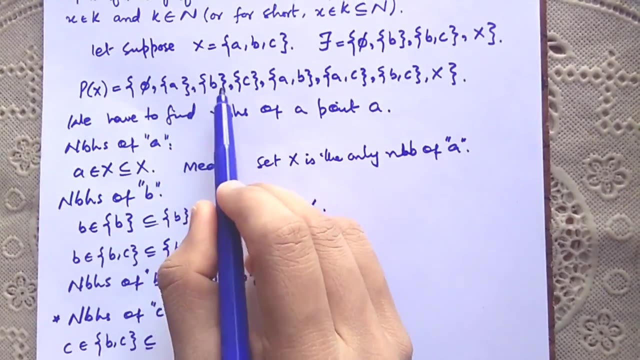 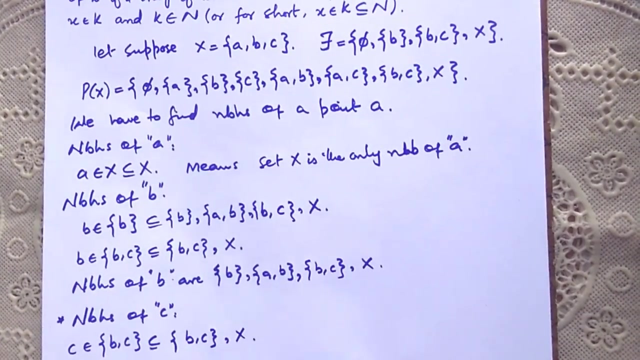 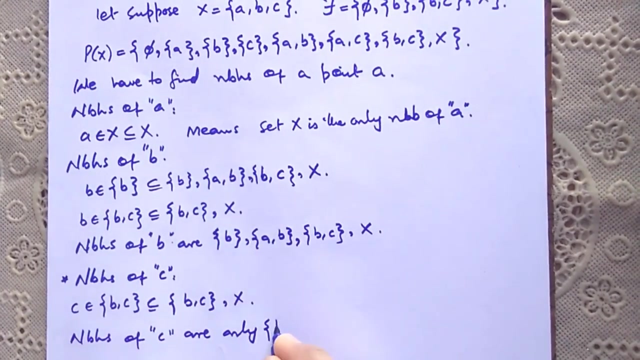 Right, Right. So for C there exists a open set, BC, such that C belongs to set BC, and there are subsets of a ground set X, such that BC is the subset of those subsets. So BC is the subset of only BC means itself and X, So neighborhoods of C are only BC and X Right. 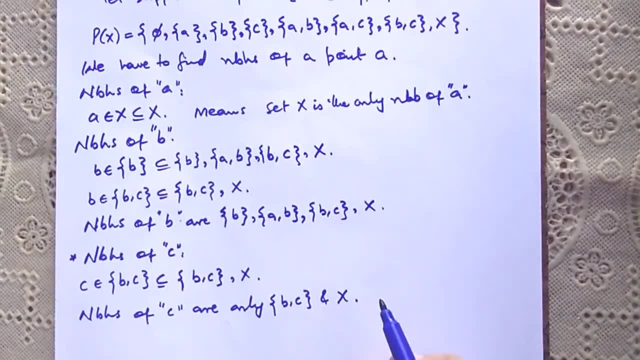 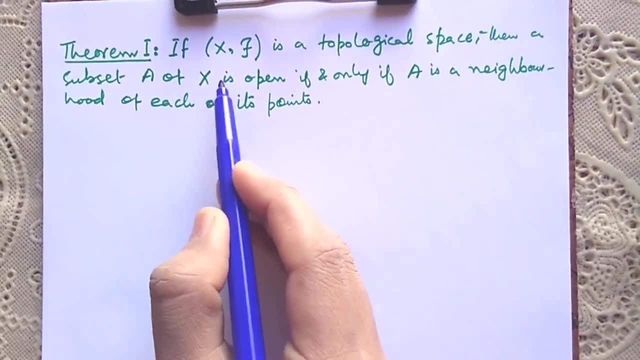 Now let's see an interesting theorem which will be helpful in finding neighborhoods. So here is a theorem: If X, with topology tau, is a topological space, then a subset A of X is open If, and only if, A is a neighborhood of each point, of each of its points. Right, 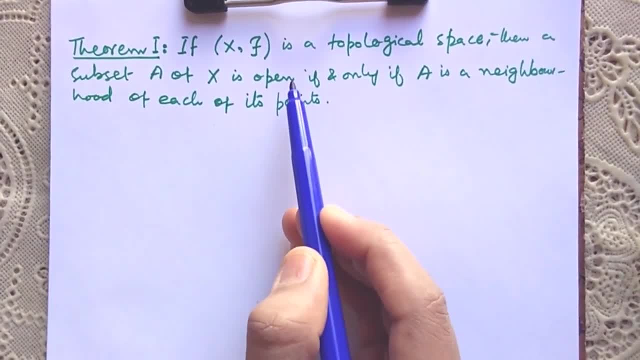 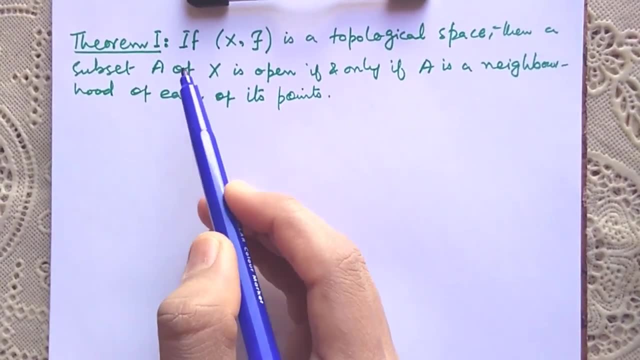 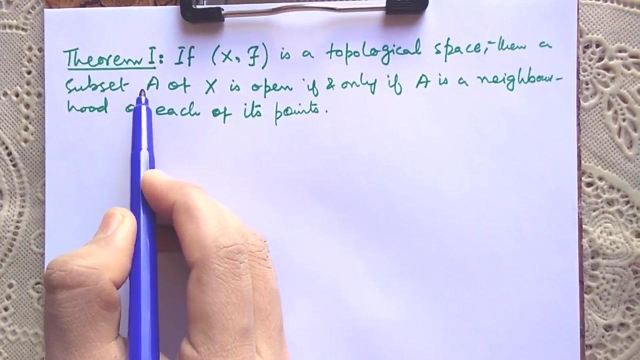 Means: according to theorem, in a topological space, subset A will be open only when subset A belongs to tau, when set A is a neighborhood of all its elements. And here if and only if condition is there means its converse is also true. Means: if every element of A has a neighborhood of set A, then set A will be open. 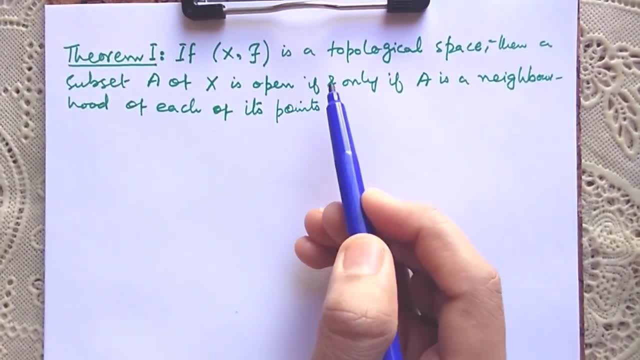 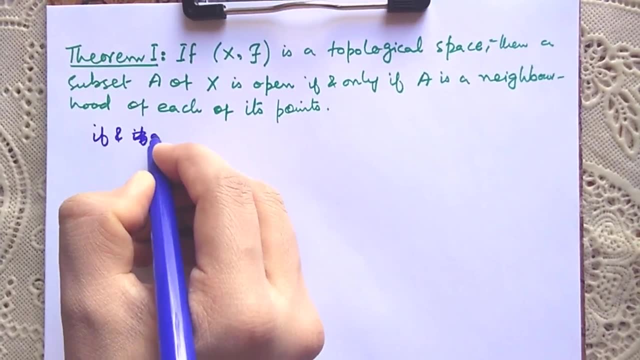 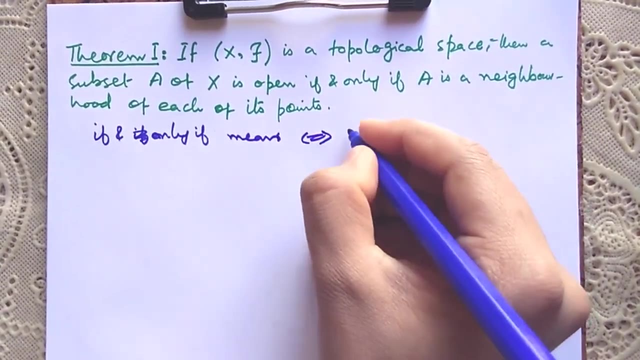 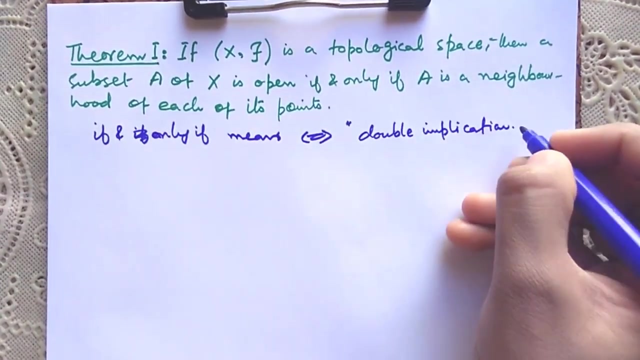 Means set A belongs to tau. Means set A belongs to tau means it will belong to tau, Right? This is its converse. And here if and only if means if and only if, means double implication, Double implication, Right? I hope you got the theorem. 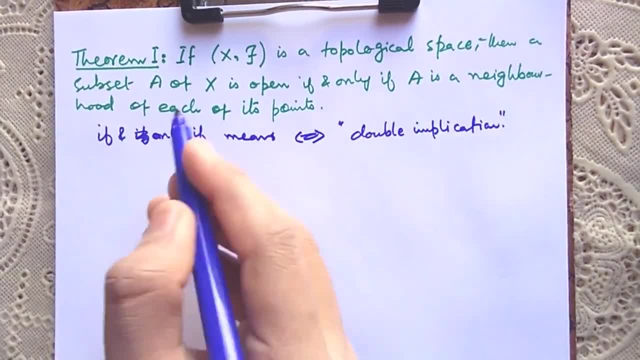 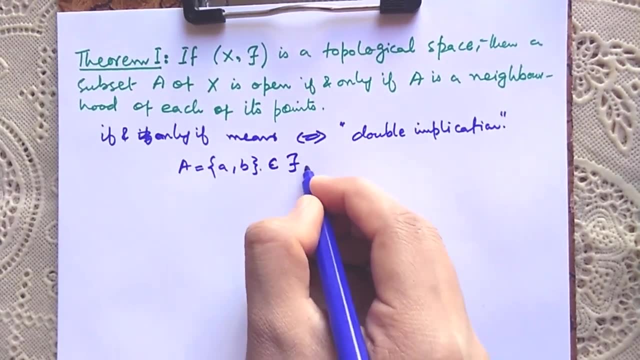 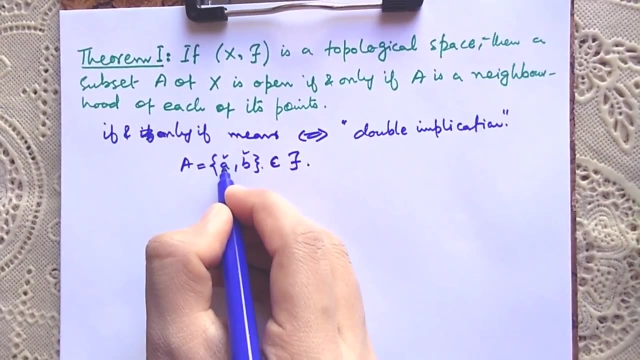 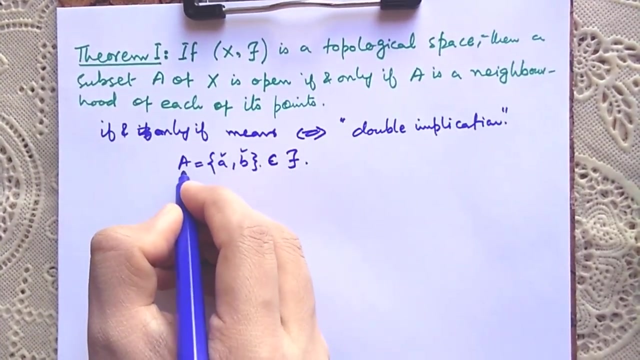 That if there is an asset, let's suppose elements of A are AB and set A is a member of Tau. so this set A and this point AB, the neighborhoods of A. you know, neighborhoods are the subsets, so one of the neighborhood of A is A. 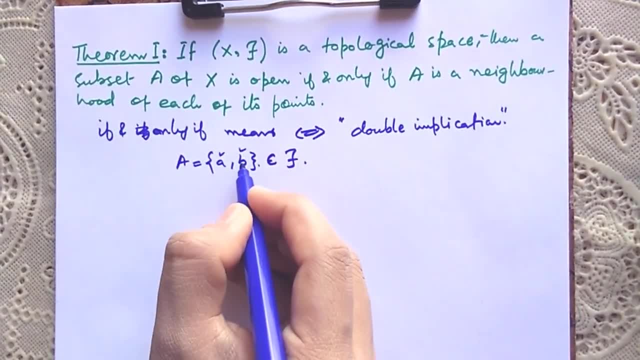 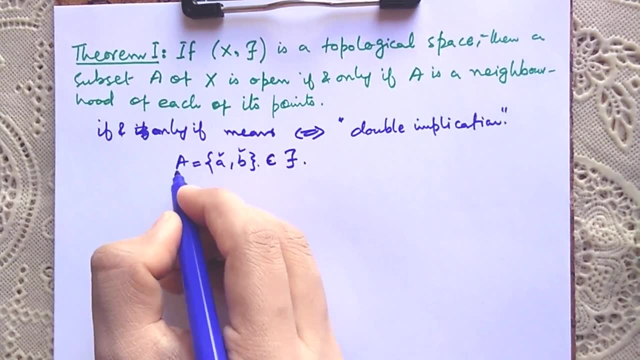 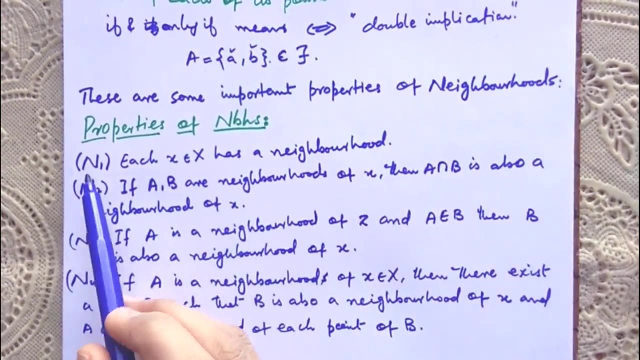 and similarly there will be a neighborhood of B. there will be a lot of neighborhoods of B and A, so one of the neighborhood will be set A if A is open, and vice versa. right now there are some important properties of a neighborhood. first one is: each x belongs to x as a neighborhood. 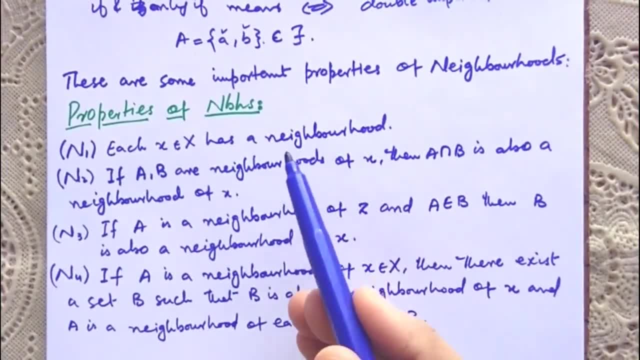 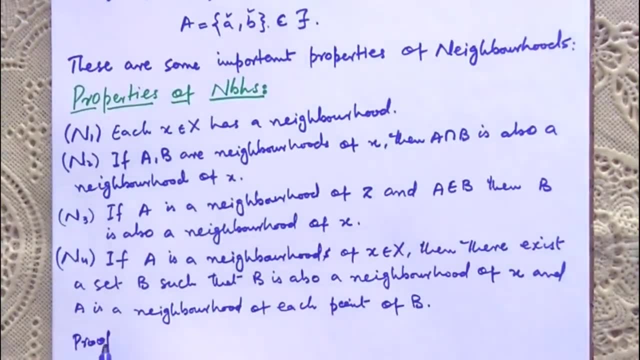 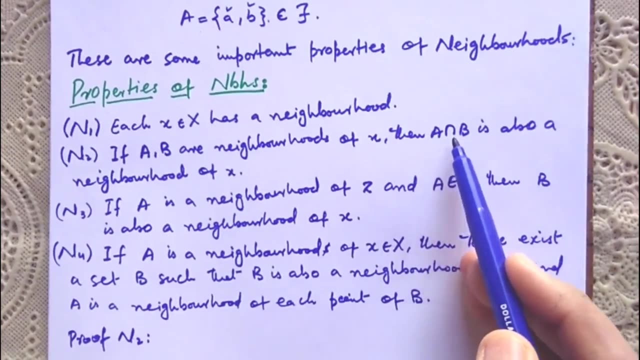 and its proof is simple because at least each point has a ground set x as a neighborhood right now. proof of 2. ok, proof of n2. and what is n2? if A and B are neighborhoods of x, then A intersection B is also a neighborhood of x. 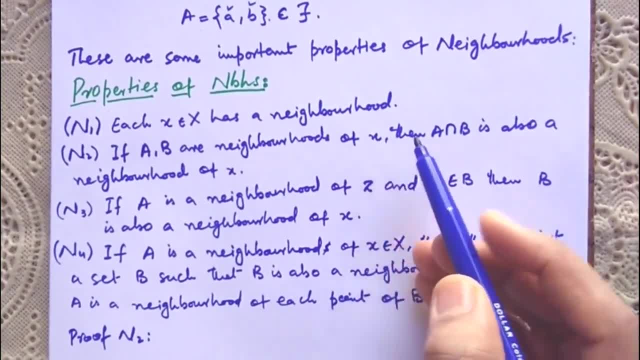 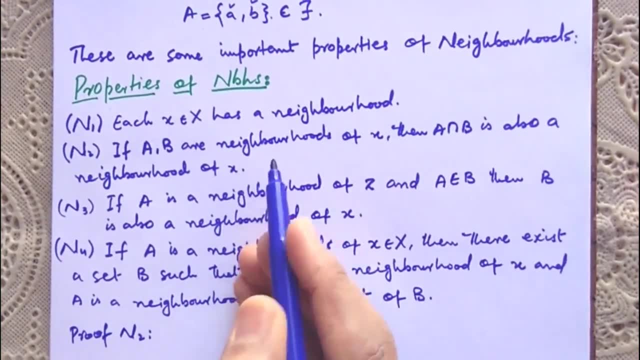 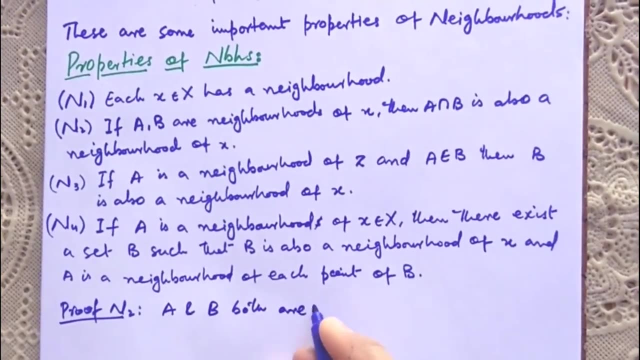 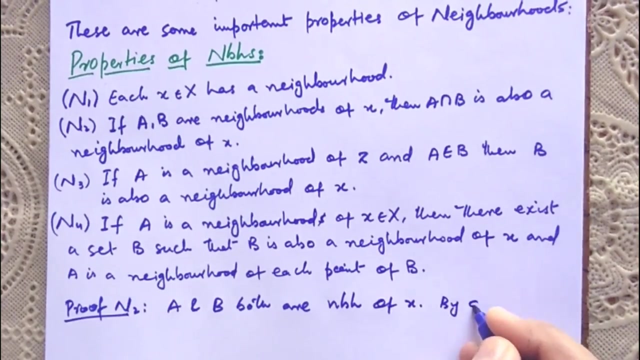 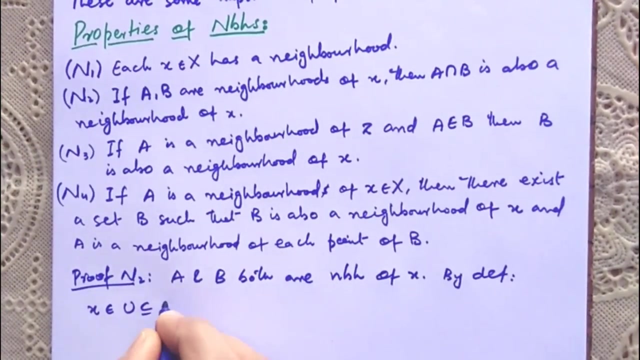 right means if these two sets are the neighborhoods of x, then the set A, intersection B, will also be the neighborhood of x, right? so let's prove this: A and B, both are neighborhoods of x. so, according to definition, by definition x belongs to U, such that U is the subset of A. 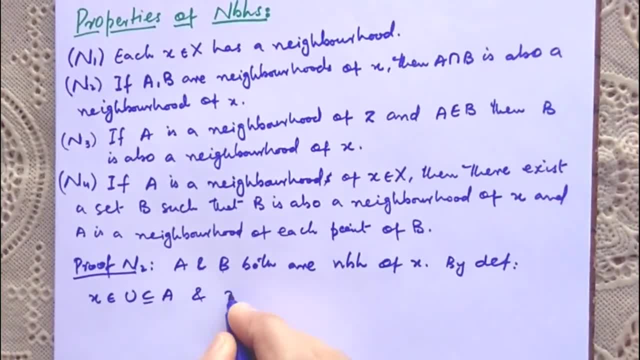 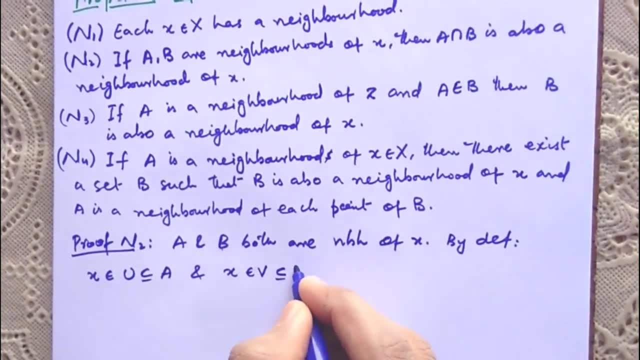 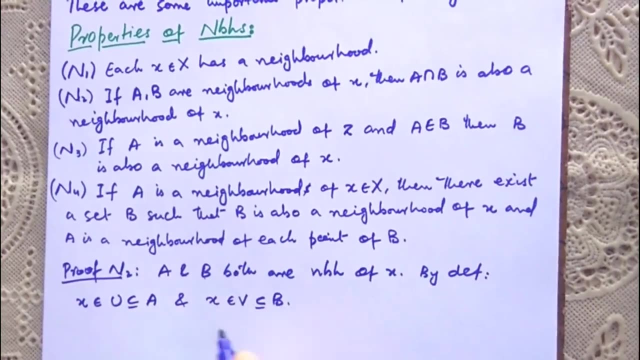 and B is also a neighborhood of x, so x belongs to. there exists an open set V, such that x belongs to V and V is the subset of set B. right now x belongs to U as well and x belongs to V as well. it means that it implies that 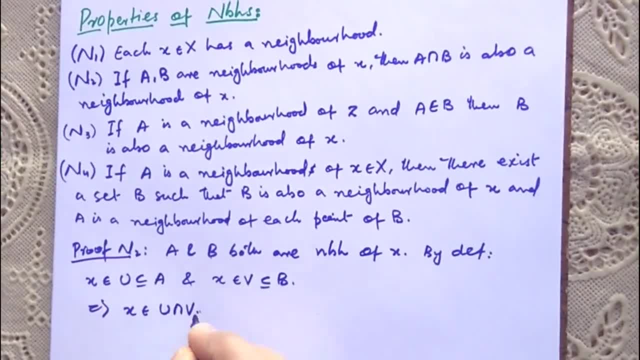 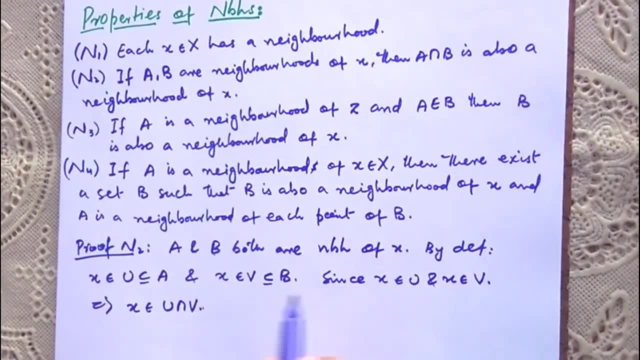 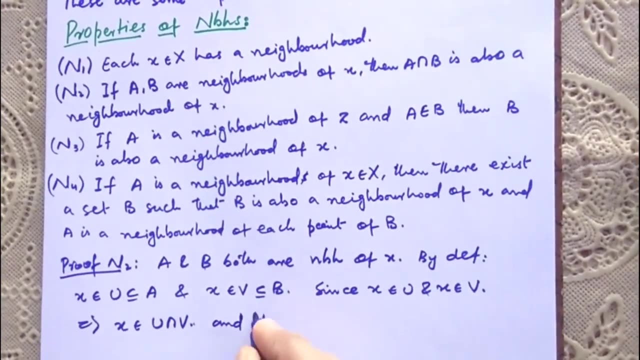 x belongs to U, intersection V right, since x belongs to U and x belongs to V. so it implies that x belongs to U, intersection V right and U. U is the subset of A and V is the subset of B, means all the elements of U are present in A. 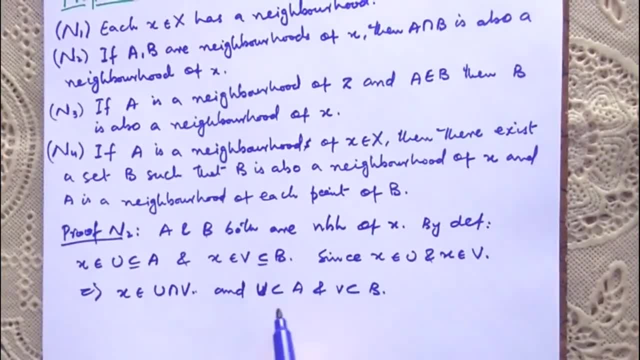 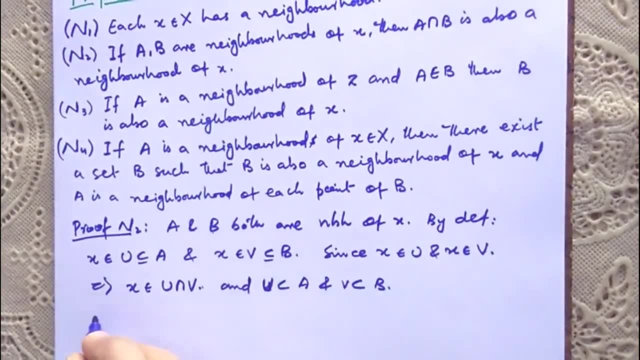 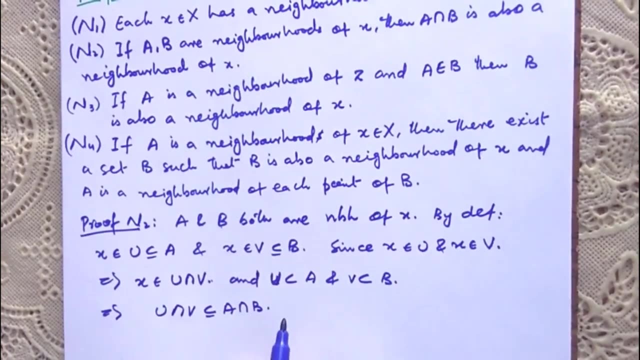 and all the elements of V are present in B. element x is common in U and V because x belongs to U intersection V right. so it means that it implies that U intersection V is the subset of A intersection B right, and you know U and V are open. 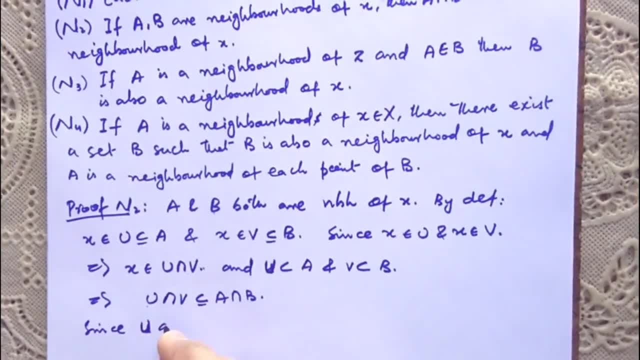 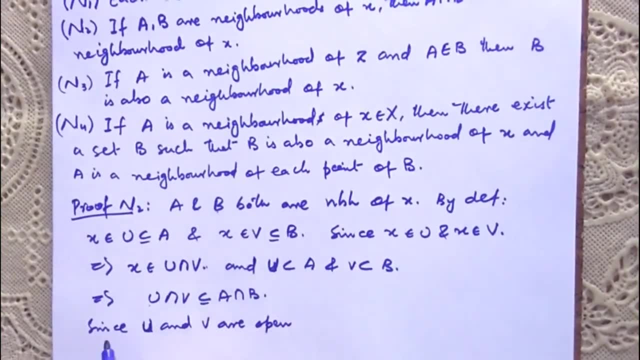 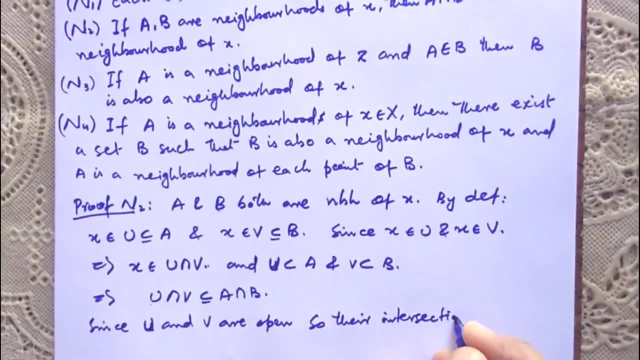 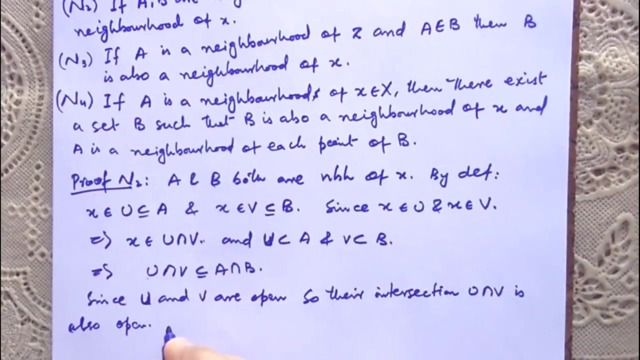 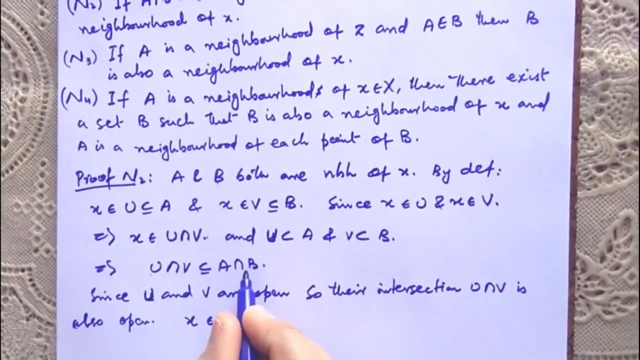 since U, U and V are open according to definition right, so U and V are open, so their intersection intersection U intersection V is also open. also open, so x belongs to U intersection V and U intersection V is the subset of A intersection B and U intersection V is open. 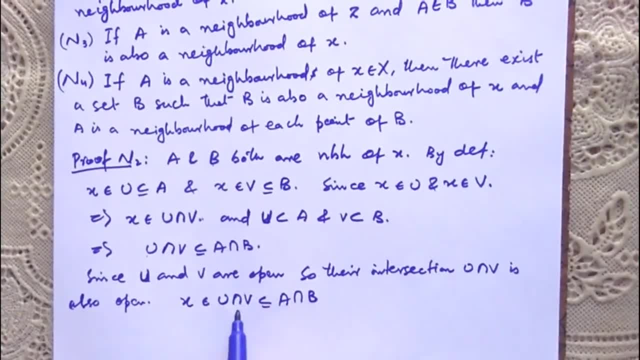 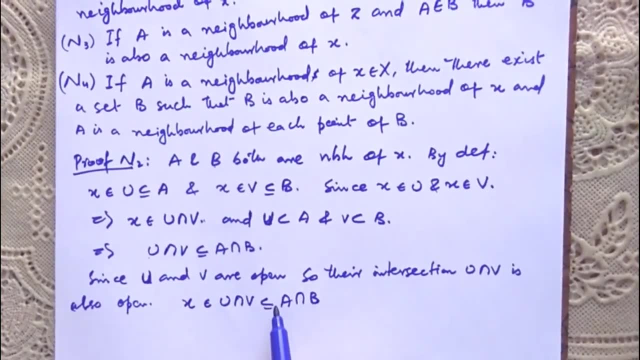 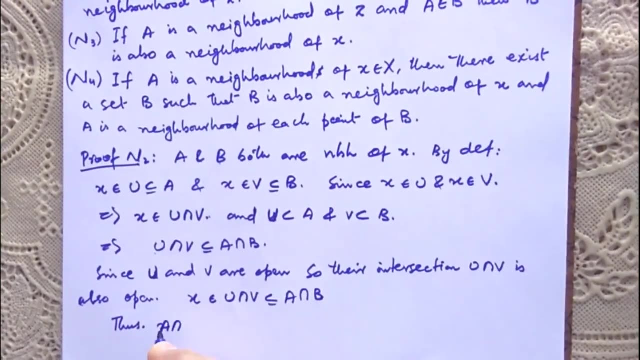 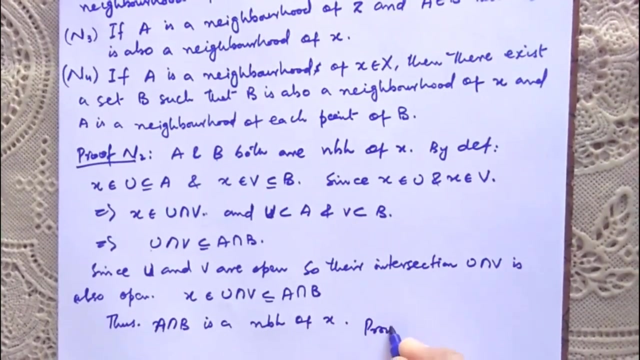 so it satisfies the definition of a neighborhood. so it means that if x belongs to U intersection V and where U intersection V is open and U intersection V is the subset of A intersection B, it means that A intersection B is a neighborhood of x, proved right now. the third property is: 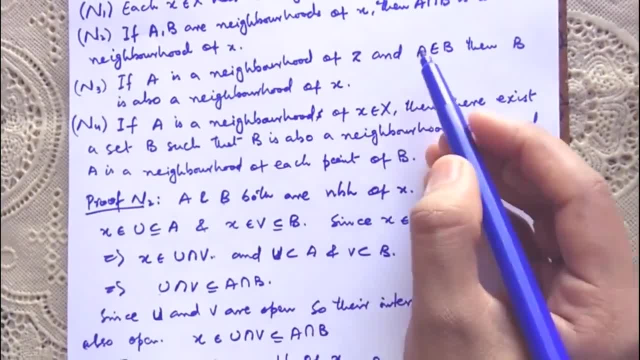 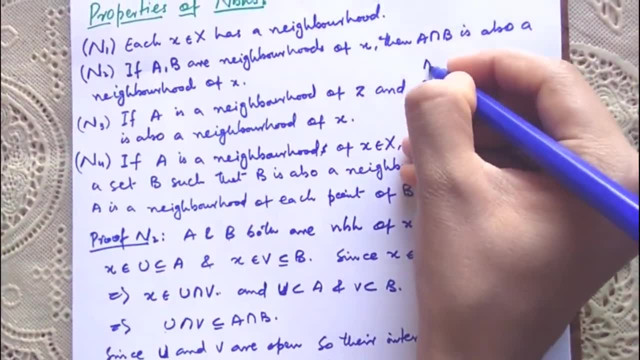 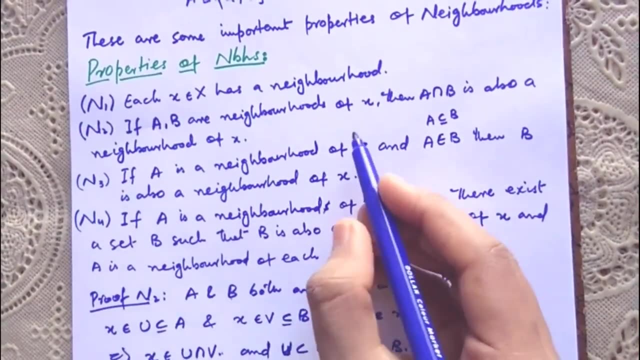 if A is a neighborhood of Z, A belongs to B- then B is also a neighborhood of x. A belongs to B. B means A is the subset of B, right. so according to third property, if A is a neighborhood of Z where Z belongs to x, then if 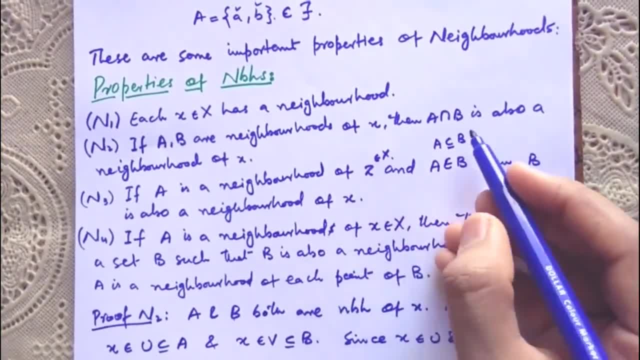 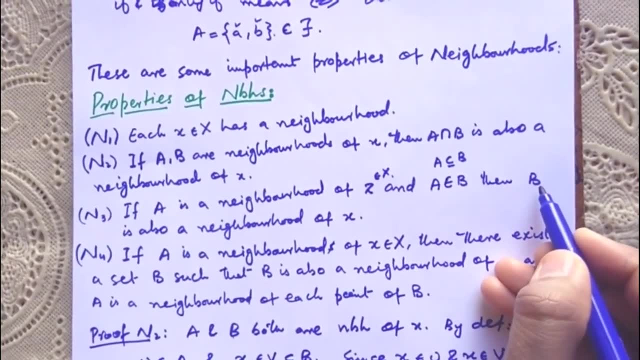 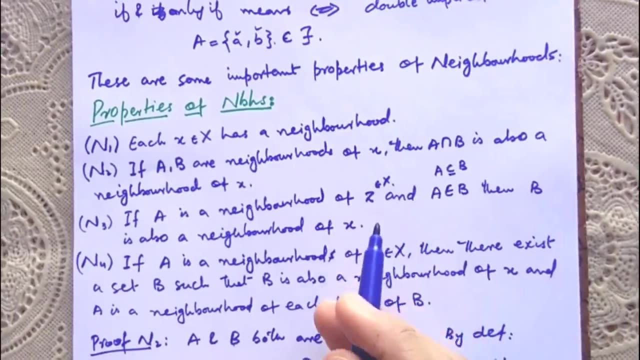 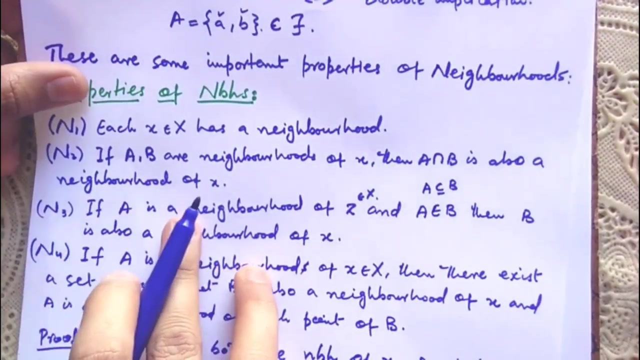 A is a neighborhood of Z and A is a subset of B, then B set, which is a superset. so this is a superset A. B is also a neighborhood of x, right? so let me prove it. proof of property 3. so if A is a neighborhood of Z, 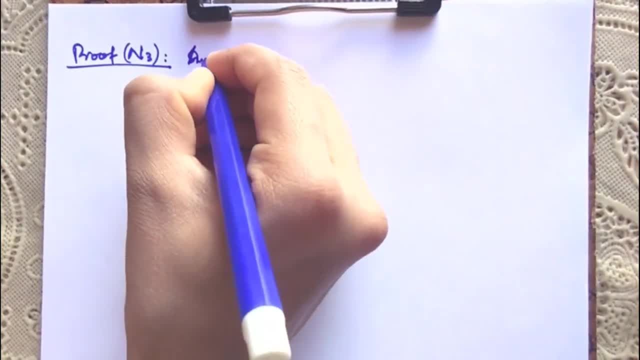 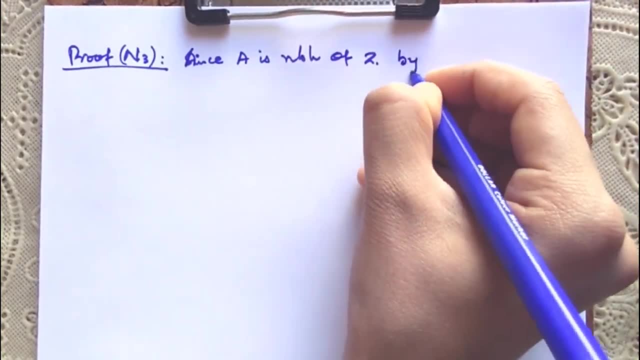 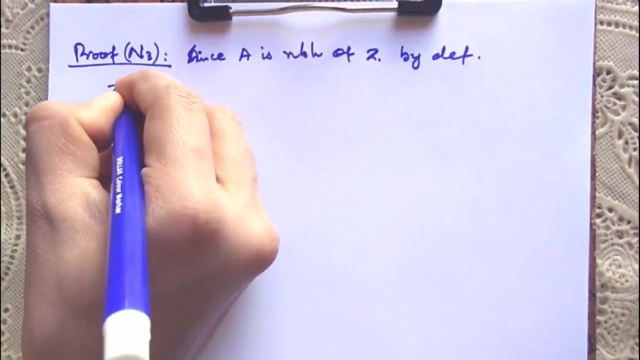 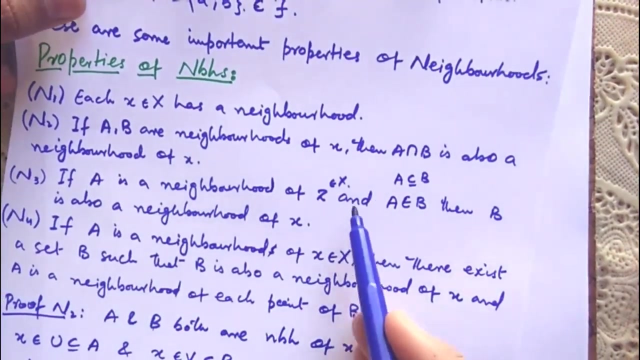 it means that A is a, since A is a neighborhood of Z. so, by definition, by definition, there exists an open set, U, such that Z belongs to U and U is the subset of A right. but, according to property, A is the subset of B. A belongs to B. 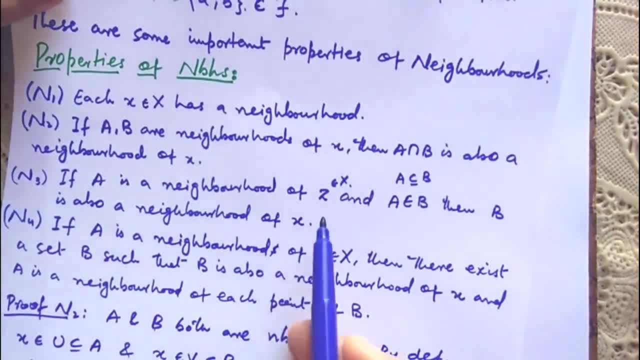 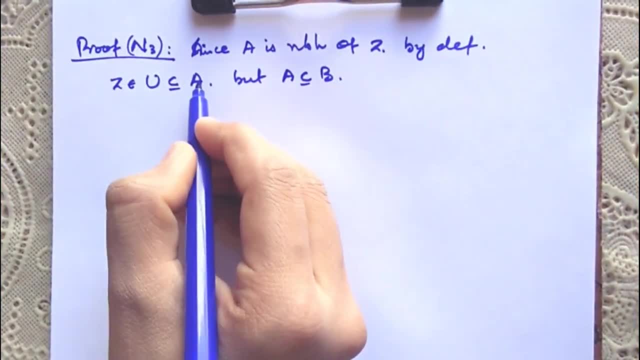 it means that A is a subset of B. then B is also a neighborhood of x, so, but A is the subset of B. so if U is a subset of A, then A is a subset of B. it means that U is also a subset of B, right? 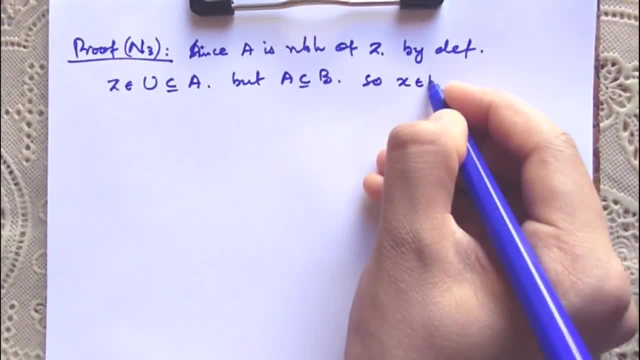 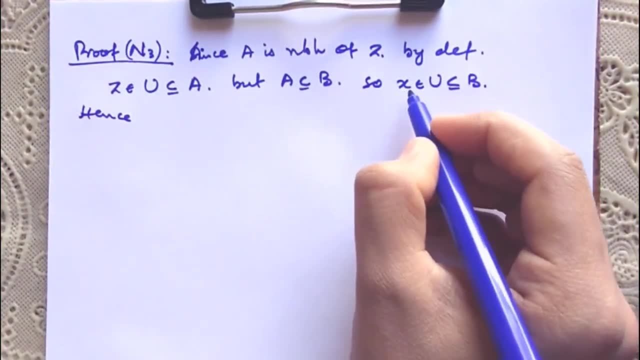 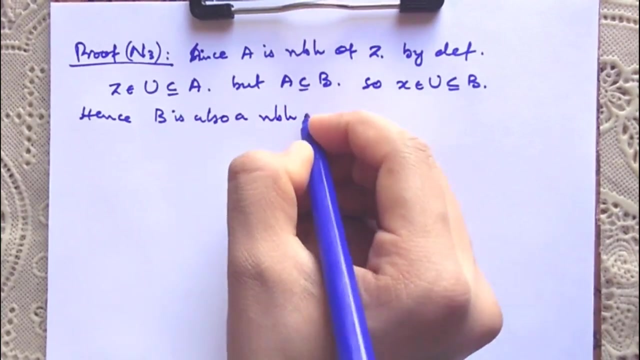 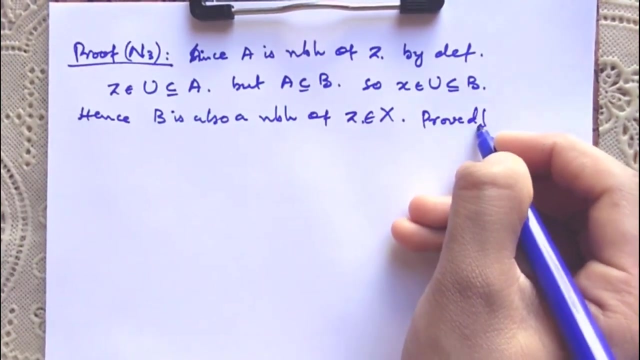 so X belongs to U and U is the subset of B, right, since it satisfies the condition of neighborhood. so B is also a neighborhood of Z belongs to X, proved right. now let's see the last property, if. if A is a neighborhood of X belongs to X. 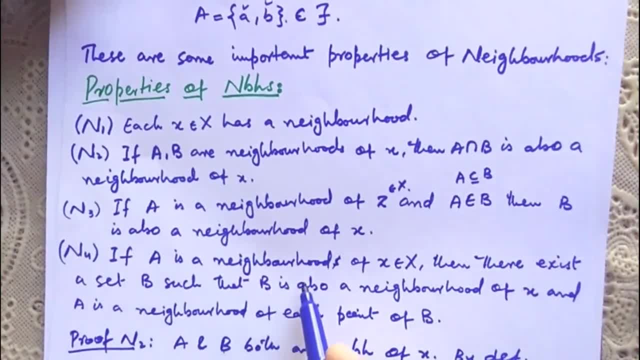 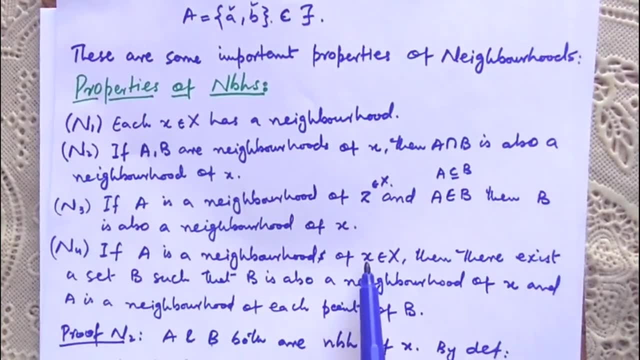 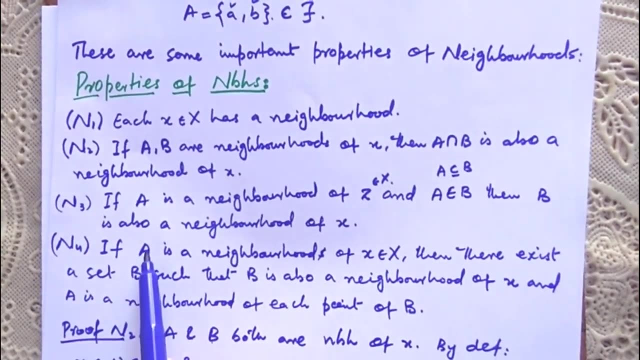 then there exists a set B, such that B is also a neighborhood of X and A is a neighborhood of each point of B. means, if A is a neighborhood of X, then a set B exists, then B is also a neighborhood of X and set A is a neighborhood of. 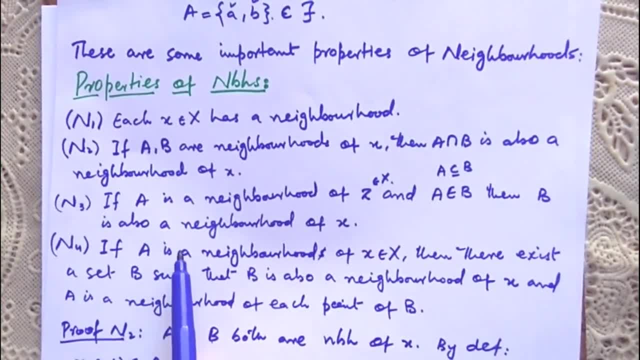 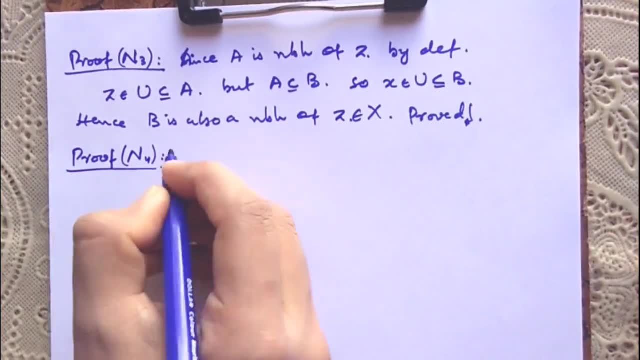 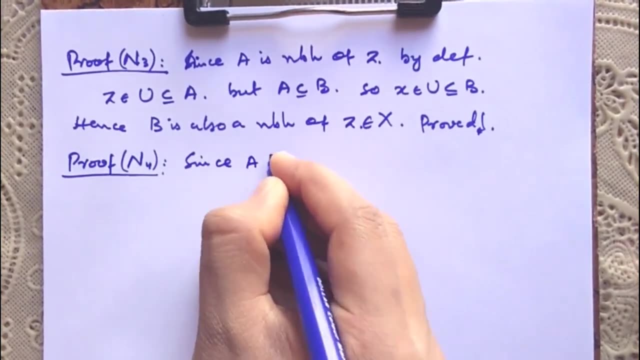 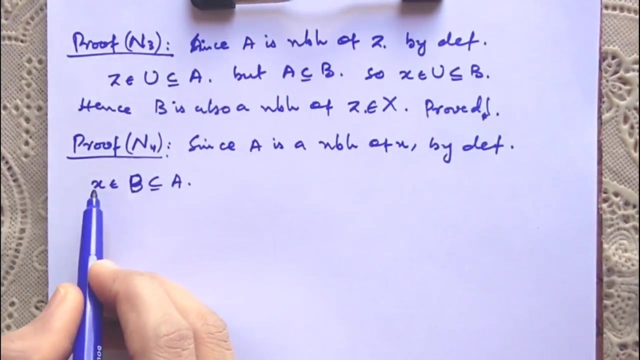 all elements of set B right? so let me prove it. proof of false property: false property. so A is a neighborhood of X. since A is a neighborhood of X by definition, there exists an open set B, such that X belongs to B and B is the subset of. 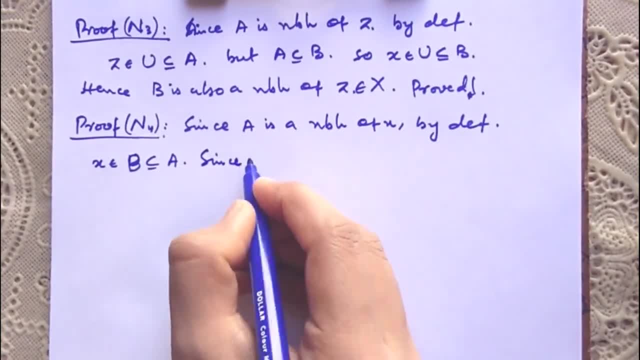 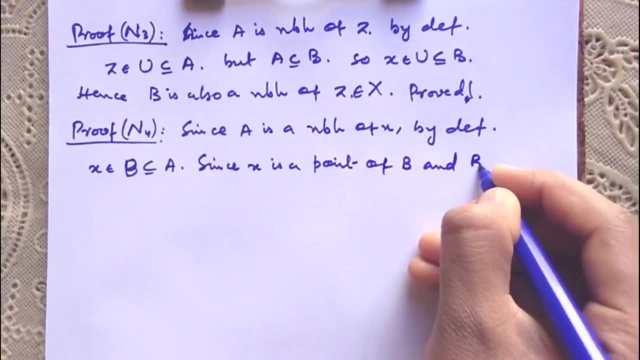 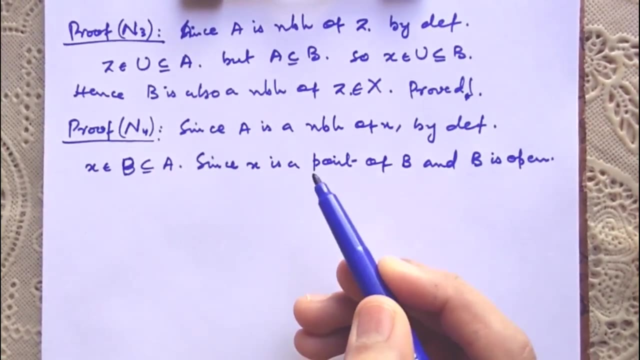 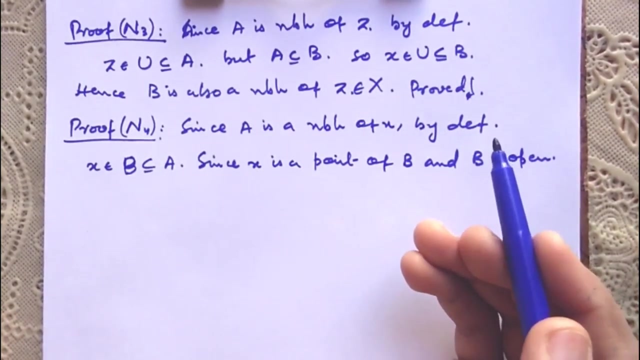 A right now, since X is a point of B and B is open, right? so now we have read the theorem, theorem 1, that an open set is a neighborhood of all its elements. so according to that, theorem B will be a neighborhood of all its elements, right? 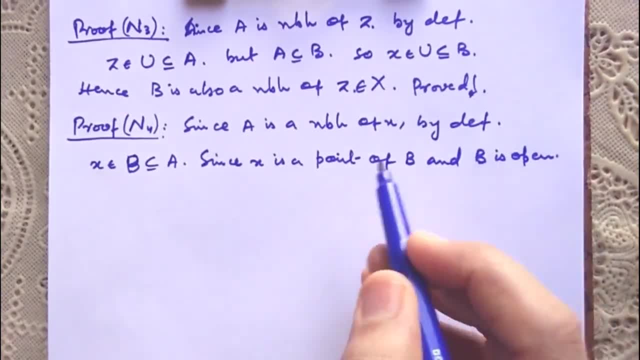 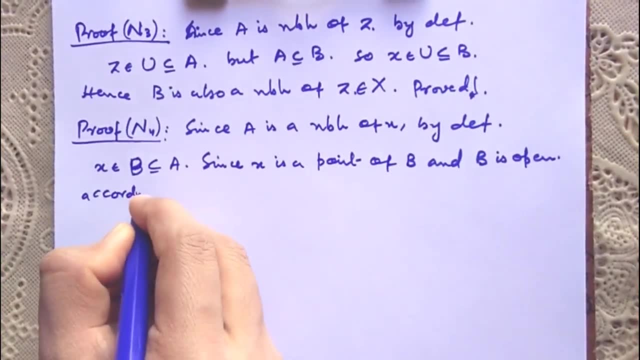 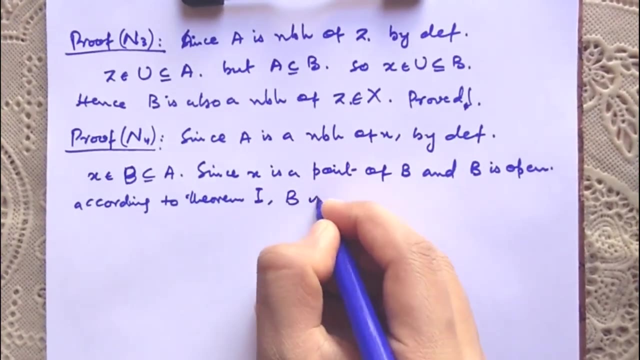 because B is an open set, so B will be a neighborhood of X, because X belongs to B. so according to theorem, B is open. so according to theorem, according to theorem 1, theorem 1: B is a neighborhood of B is a neighborhood of B is a. 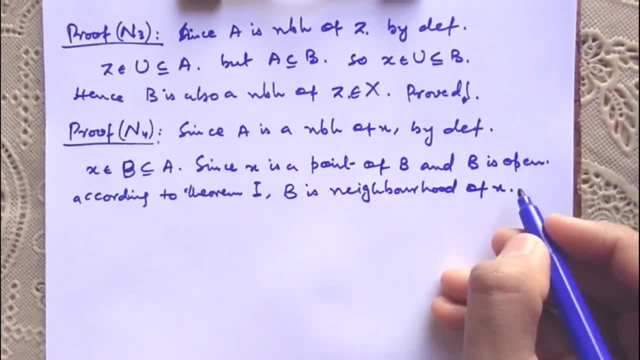 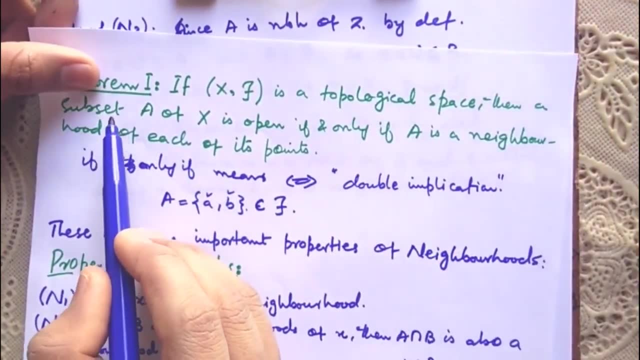 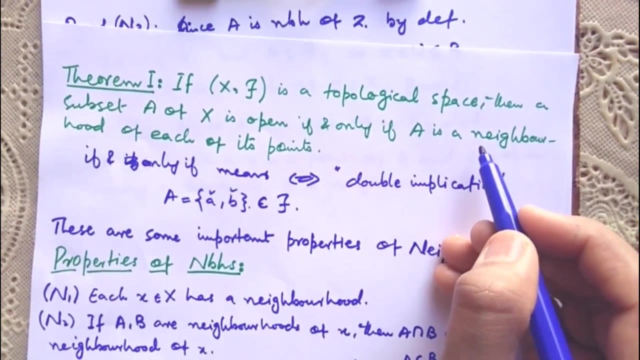 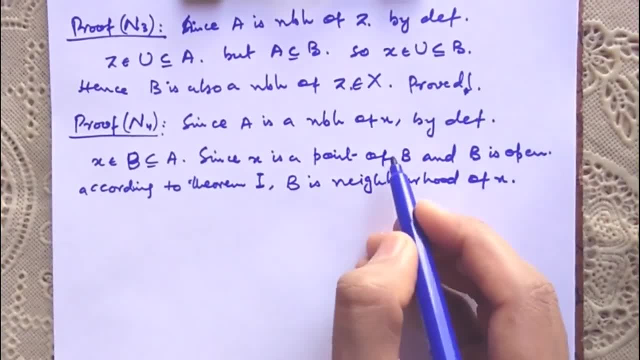 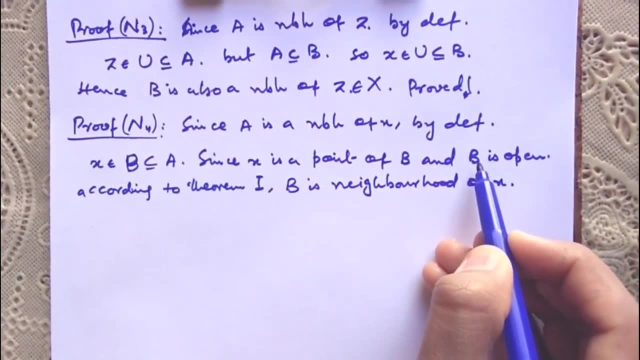 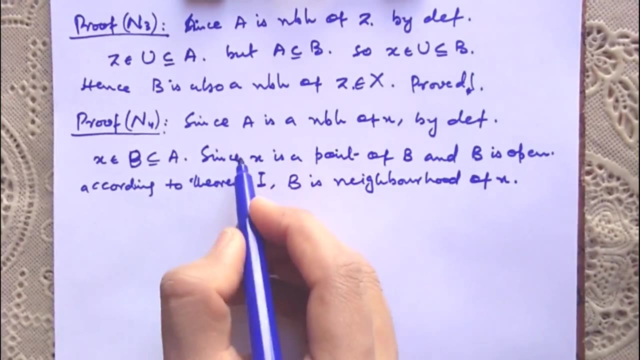 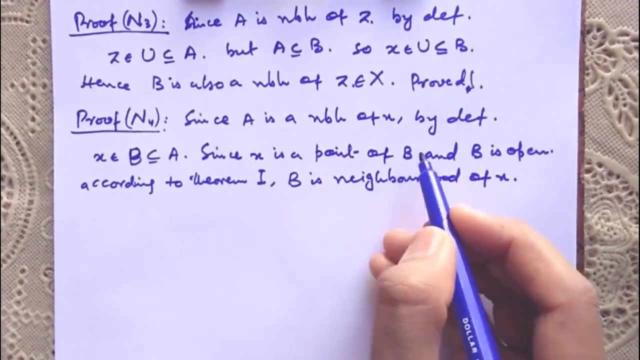 the an is open set and x is also belonging to B, it means that B is open. it means that all the elements of B, all the individual elements of B, there will be a neighborhood set B, right. so x is also an element of B because it belongs to B. so if x is an element of B, it means 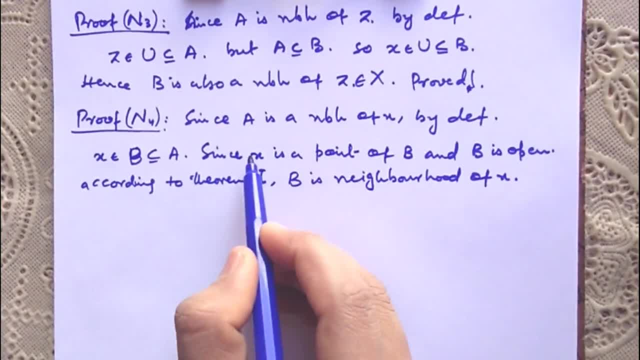 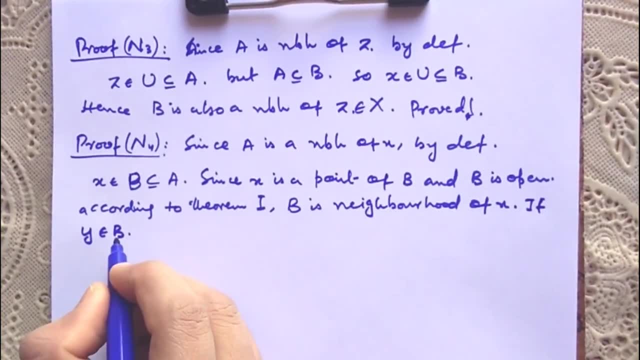 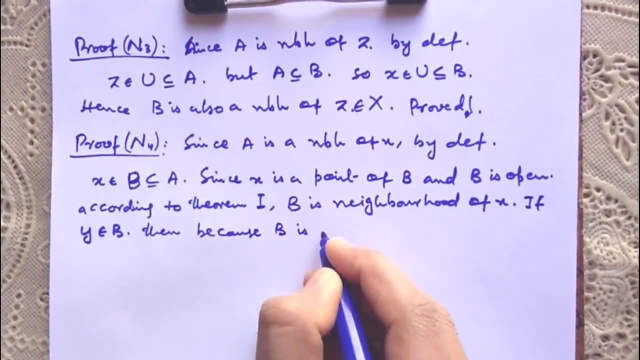 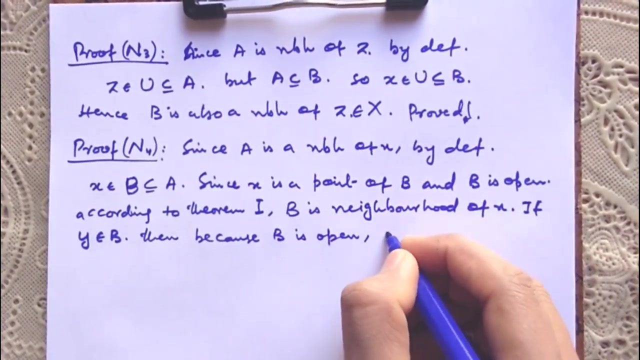 that B is a neighborhood of. according to theorem, B is a neighborhood of x. right now, if y belongs to B, there is another element, y, that belongs to B, then, because B is open, means B belongs to tau. so, again according to theorem. again according to theorem 1. 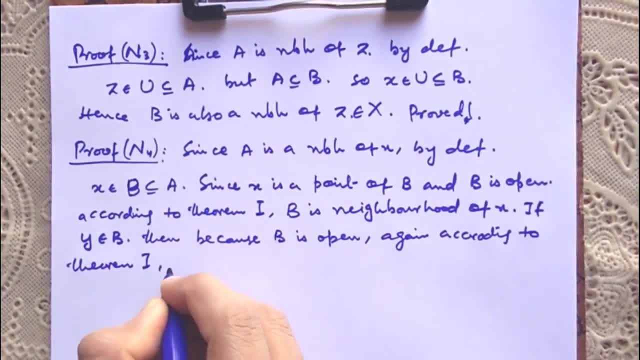 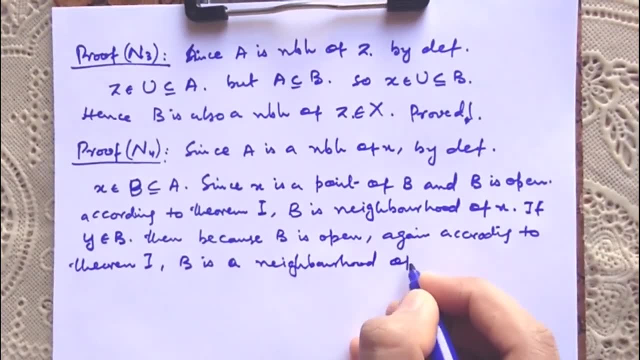 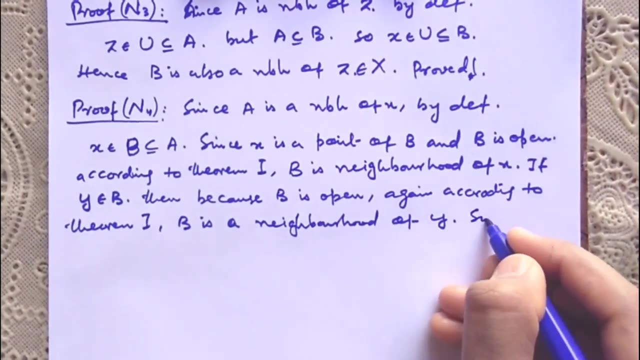 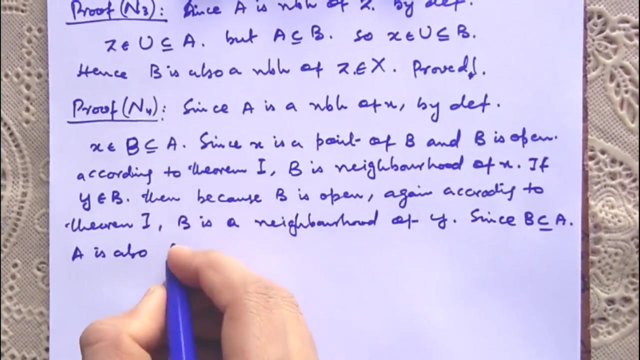 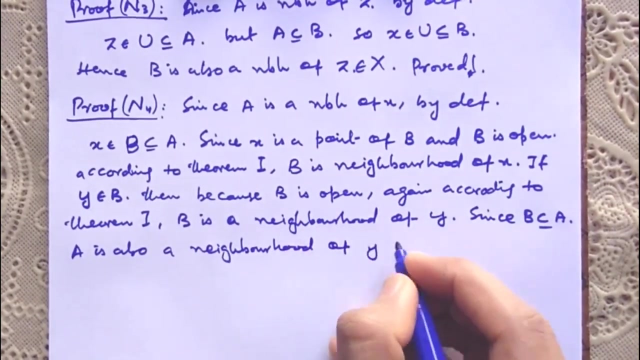 according to theorem 1, B is a neighborhood of y. right now, by definition of the neighborhood, B is the subset of A. since B is the subset of A, so A is also a neighborhood of A is also a neighborhood of B, neighborhood of B neighborhood of y by property 3, because third property says that if A is a neighborhood, 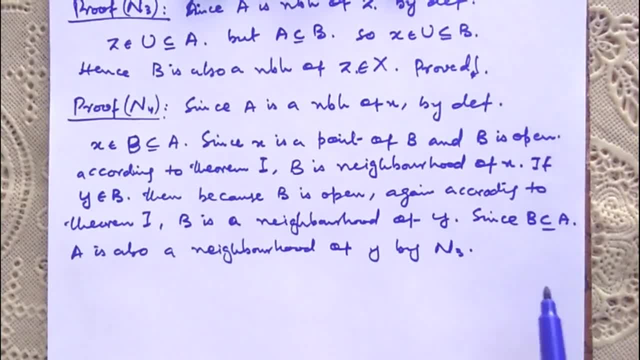 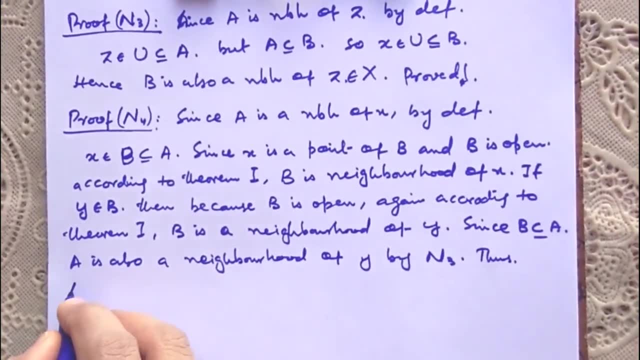 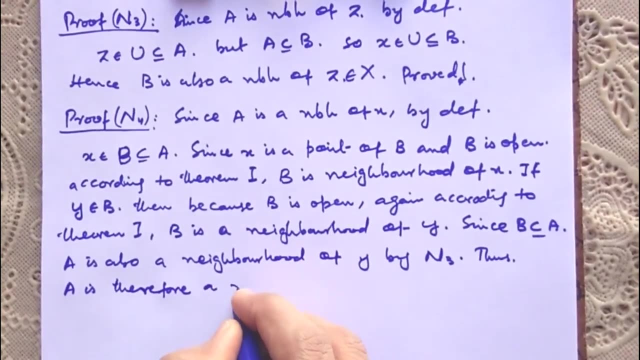 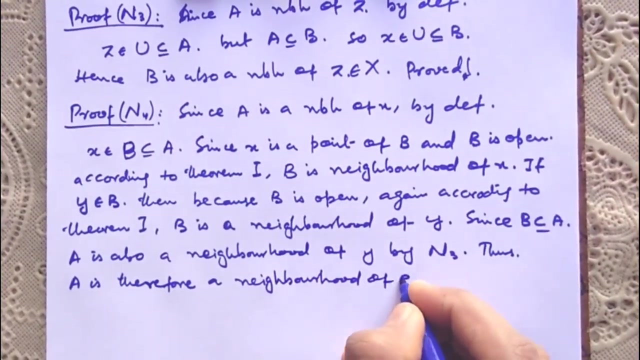 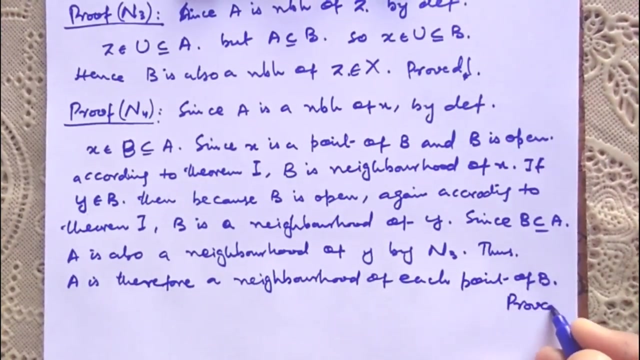 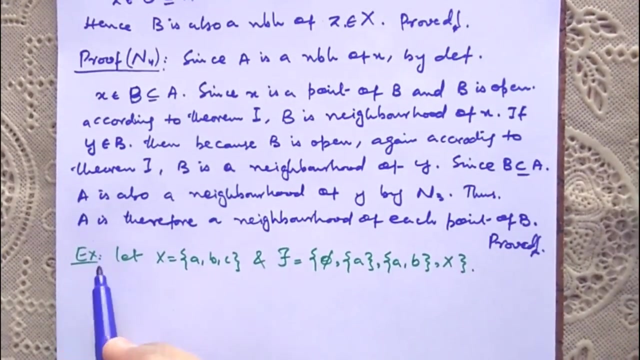 of x and A is the subset of B, then B is also a neighborhood of x, right? so here is the same situation. thus, A is therefore a neighborhood, a neighborhood of x. now let's determine the set of B by using above properties. so here is an example. let x be the set of three elements and there is a topology tau. 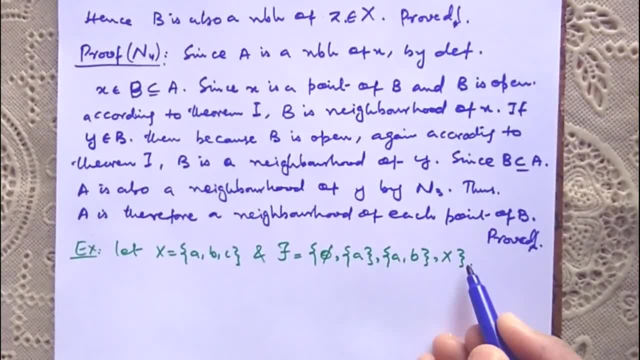 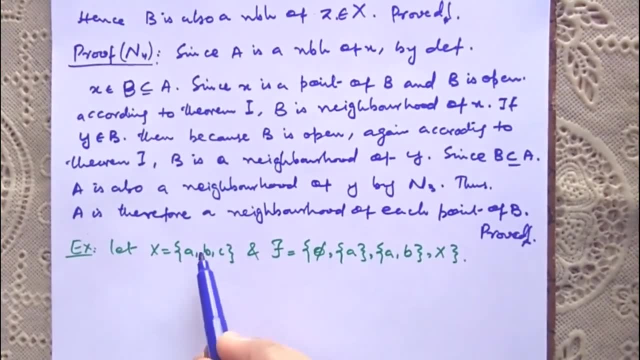 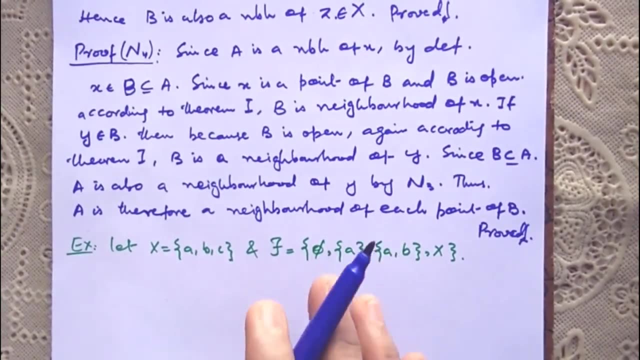 that contains phi set A, ab and x. right now we have to determine the neighborhoods of A, B and C, So let me write the neighborhoods in the form of neighborhood system. Neighborhood system means writing the neighborhoods of any point x0 in a set Right. So neighborhoods. 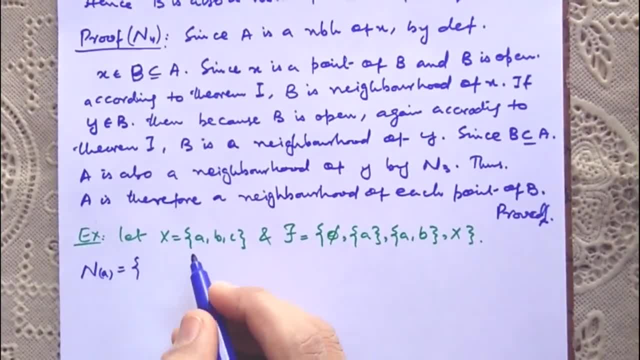 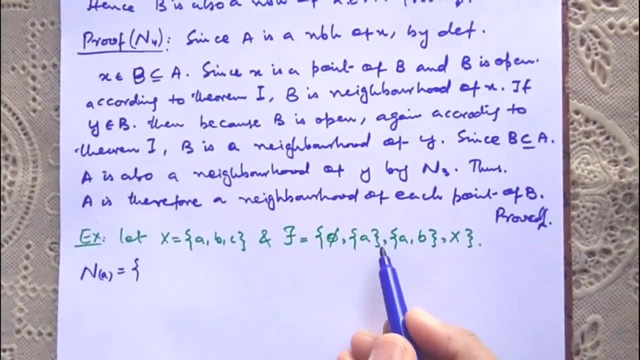 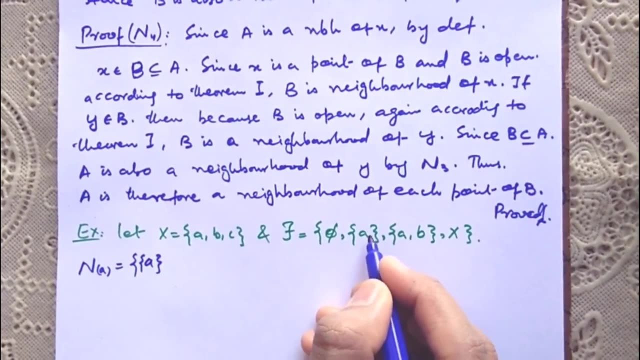 of A. Now for A. first of all we will see the open set, and here A is the open set. Now apply the theorem that every open set is a neighborhood of its points Means A is an open set and this open set is a neighborhood of its points. So A is a neighborhood of. 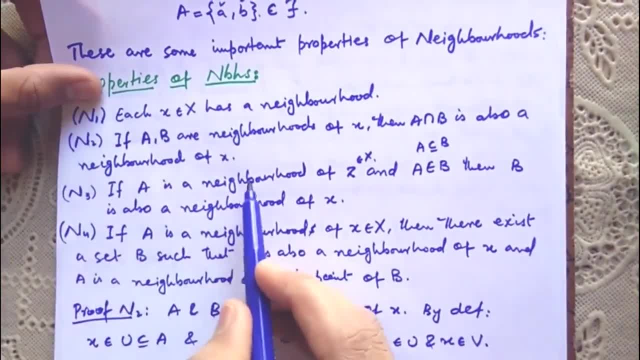 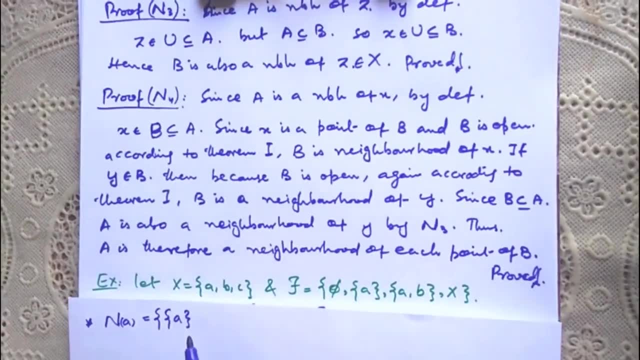 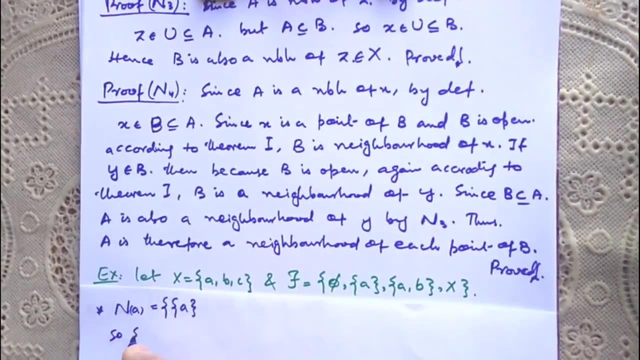 A Right. Now. according to property 3,, if A is a neighborhood of Z that belongs to X and A is the subset of B, then B is also a neighborhood of X. So other neighborhoods are those subsets of X which are superset of A Right. So A, B is a superset of A and